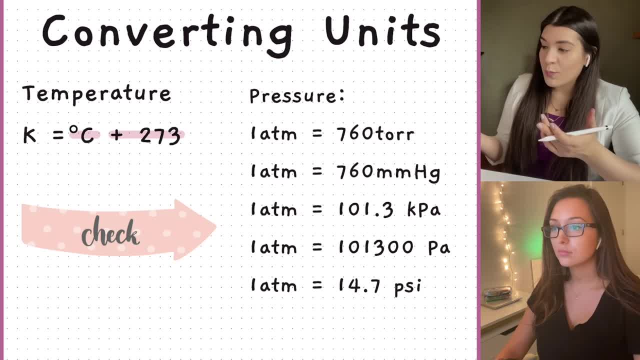 either going to specify- you know what pressure they, what unit they want in pressure, or you kind of have to pick and just see if you want to convert it back to one of them, And then you're going to see if you want it both, if you want both pressures to be in atmospheres or tor or so on. 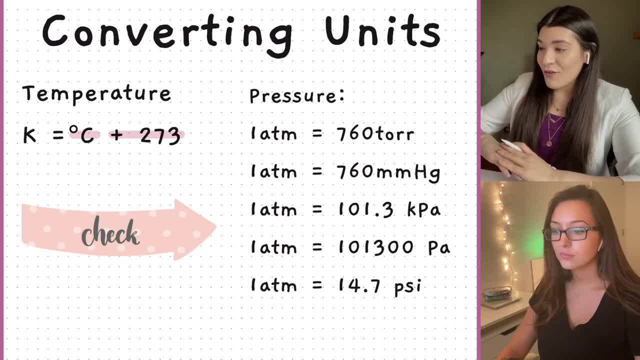 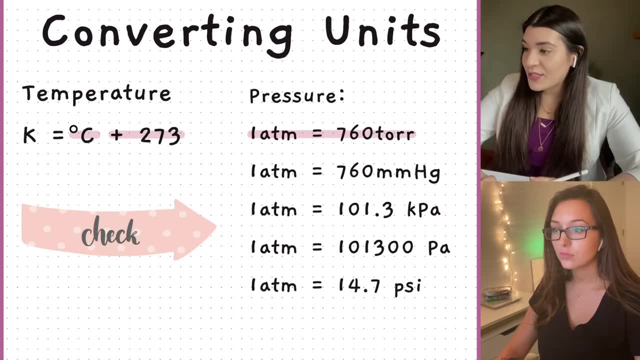 So this is all the possibilities that I typically see for pressure. This is kind of based on just the most common ones. So the most common ones is just knowing that one atmosphere is equal to 760 tor, one atmosphere is equal to 760 millimeters mercury, And then the other ones I'd say, aren't. 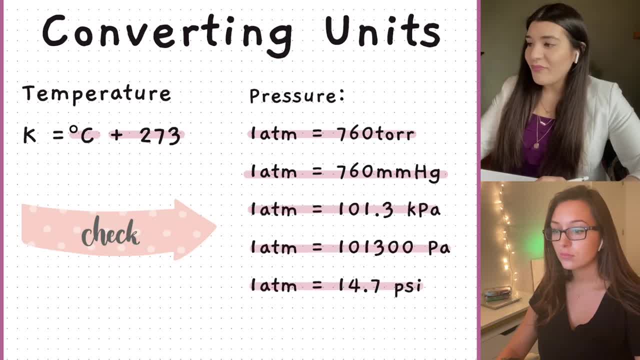 as common, but, just in case, still something to know. but we'll go back to it. We'll do several examples. Just want to cover all of our bases here, since you're starting to find out a little bit more about gas laws And then we'll finally see gas laws Now. question so far. 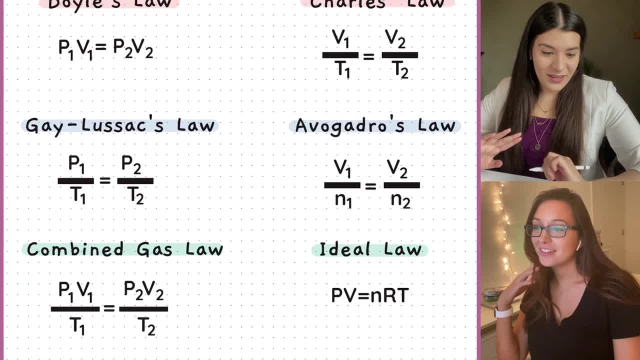 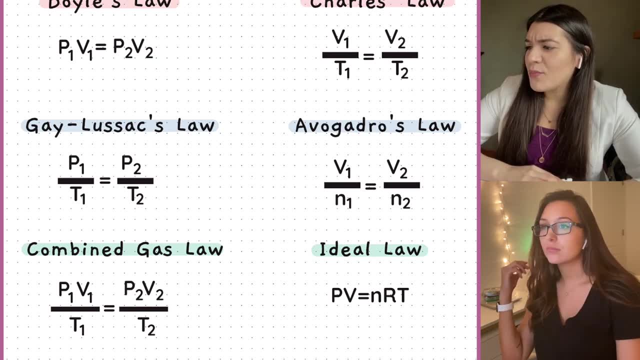 No, no, I've actually seen a little bit of this already in lab, So that's good, Okay, Perfect, I'm glad. Okay. And all of the different gas laws that you'll need to know. So these are, I'd say, the main ones. You probably will go over partial pressure as well. Dalton's. 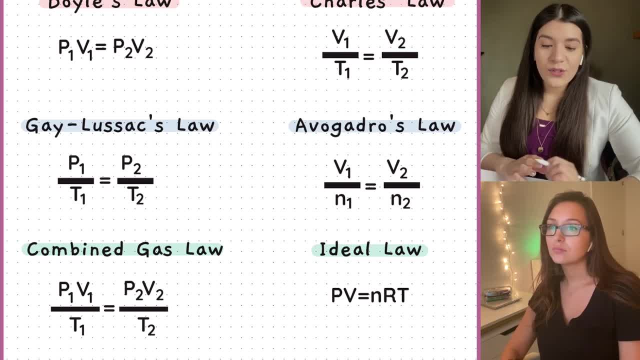 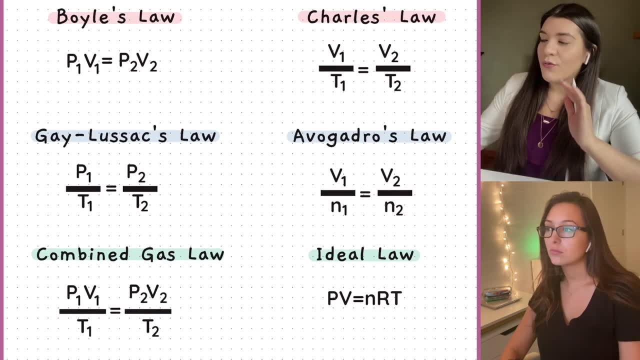 law, partial pressures, but this is like the main ones that we start off with for gas laws. So the first one is going to be Boyle's law And that's really just talking about. I'll highlight here, just. it's basically just, you know, referring to pressure and volume. 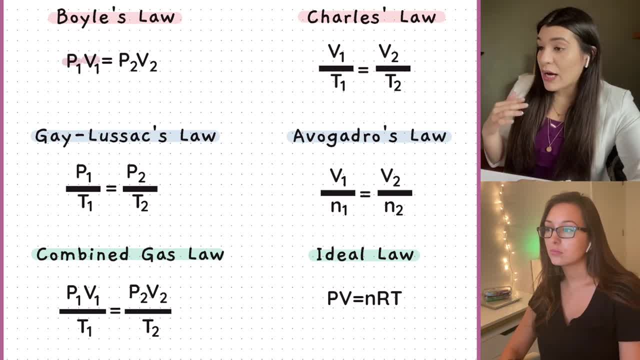 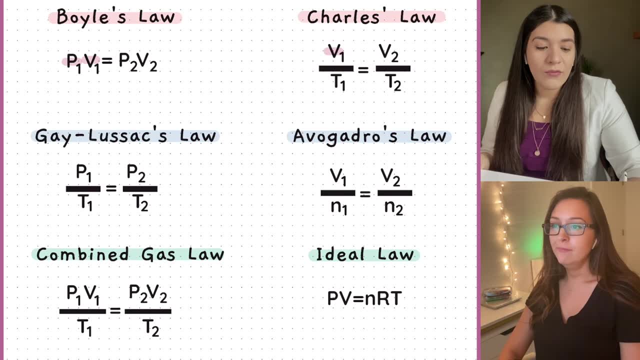 So we don't care about temperature or moles, Those are held constant. We're specifically just looking at pressure and volume. Next, with Charles law, that's something a little bit different, where we're now comparing volume and temperature, And then the next law is just comparing pressure and 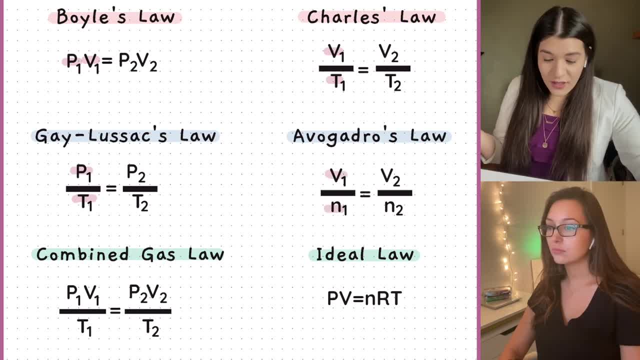 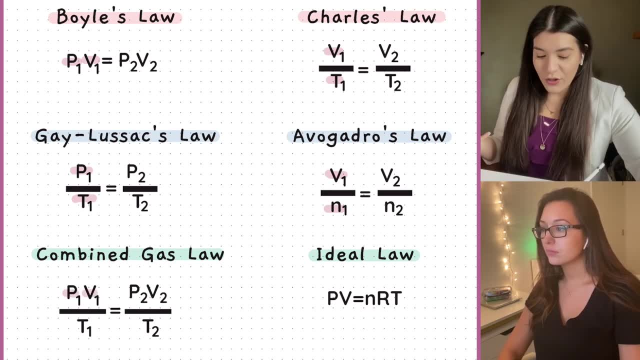 temperature of a Gaudreau's law, volume and moles, And then the combined gas law, which I know tends to be pretty tricky because you're putting everything together, So you're comparing pressure, volume and temperature, And the last one that's a little bit different from the other ones. 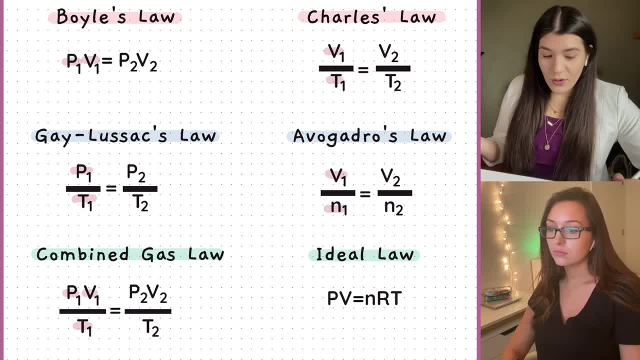 is the ideal gas law which compares basically everything. So it has pressure volume, N is our moles, R is a known gas constant that will be provided to you- Typically that's provided to you- and then temperature. So I just say this is like the main ones that I would have. 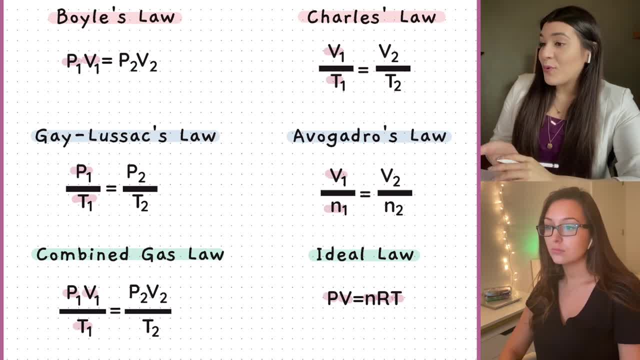 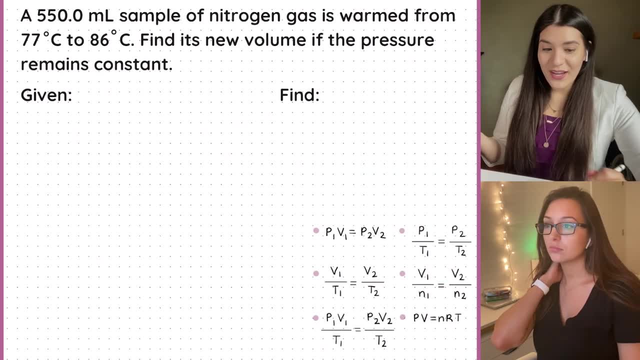 memorized. You know you have to have down to be able to answer any of these questions. So, that being said, I obviously don't expect you to know them right now. So I do have a little cheat sheet on the bottom, just so we can pick. 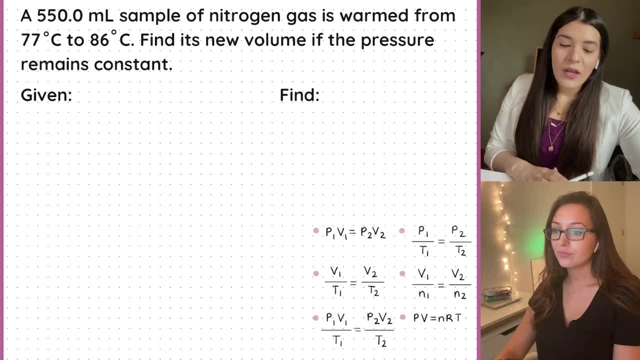 from which one like what gas law we're actually using. So how I want you to start off these questions is just like we've done before, where we have our given, we write down our given and what we're finding, And by doing so, that's literally going to tell us what formula we 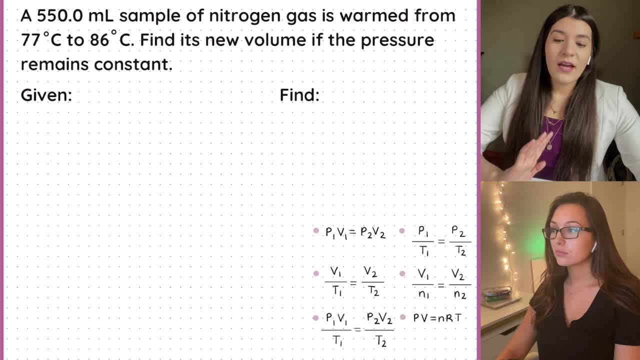 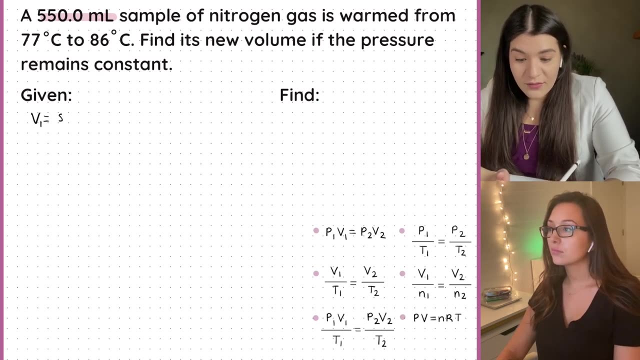 should use. So we are set to have a 550 milliliters sample. So right then, and there I can see: okay, that is a unit for volume. So since I know my first volume- okay, I know that's V1- is 550.0. 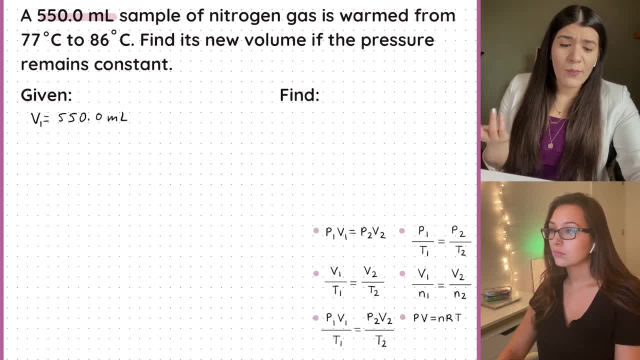 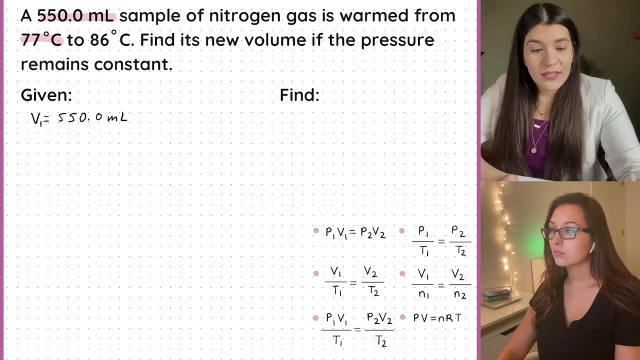 milliliters. Next, I'm going to keep going and see. okay, a sample of nitrogen gas is warmed from and it's giving me two different temperatures. So my first temperature is T1.. So that's 77 degrees Celsius, And then my second temperature is 86 degrees Celsius. 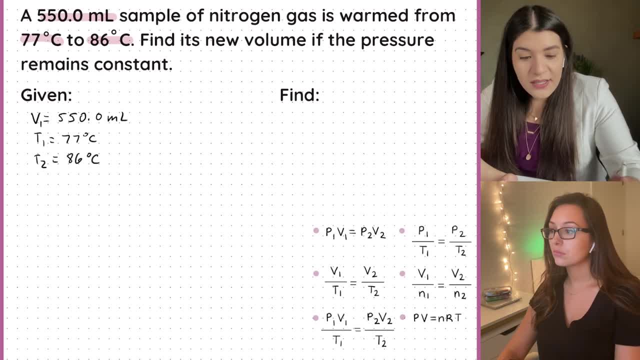 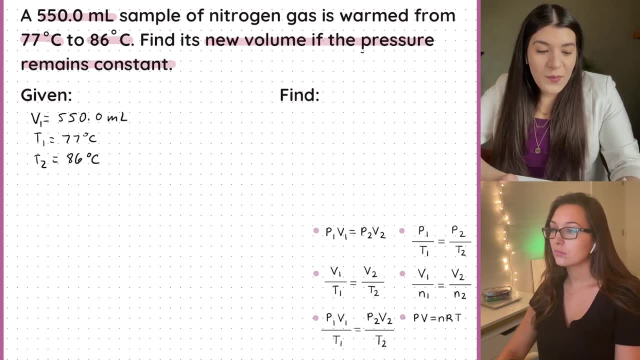 T2.. So 86 degrees Celsius. Next is telling me: find the new volume if pressure remains constant. So by them, even talking about pressure it's irrelevant, because it's held constant. That just means it doesn't do anything. There's no change, We don't have to worry about it. 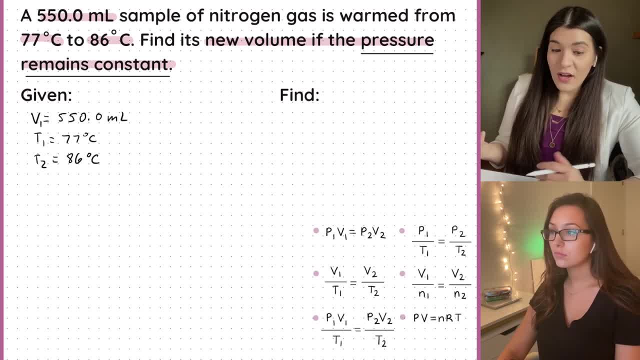 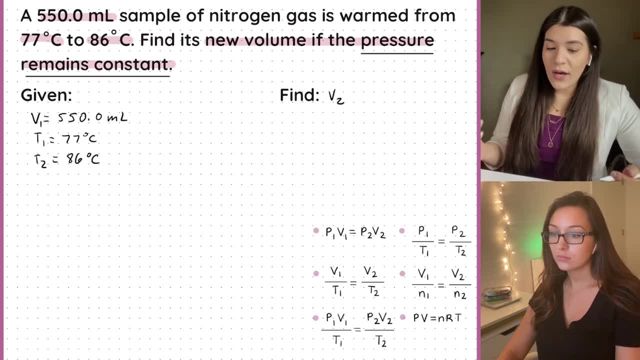 And they're not even talking about, you know, moles. We don't have to worry about that either. The only thing that they're telling us is: well, we want to find our second volume. So I'd go back to my formulas and I'd see. well, what compares? only volume and temperature. 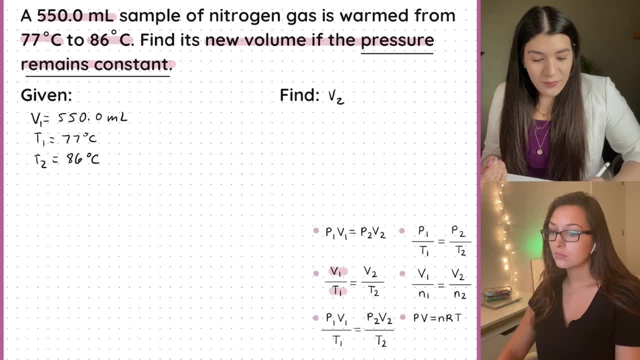 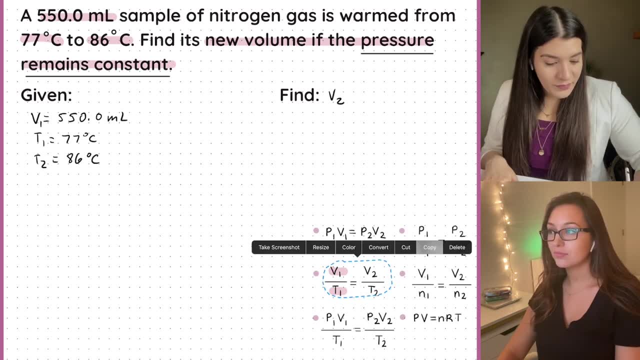 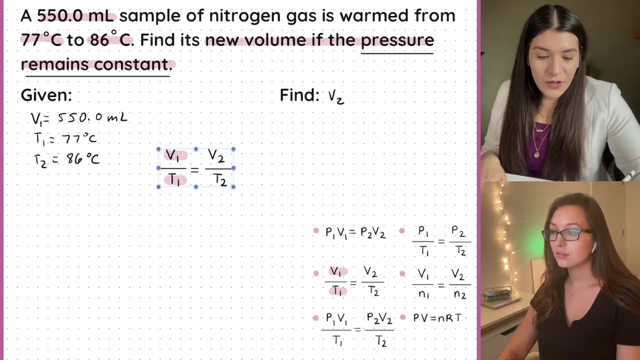 well, it has to be this one. So volume and temperature. So I know I have to use that formula. Makes sense. Yeah, Yeah, I'd say the hardest part is just memorizing them all. It's just knowing which formula. So it's, I wouldn't say it's you know. 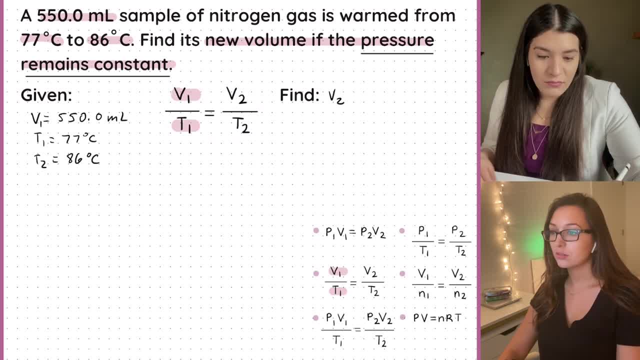 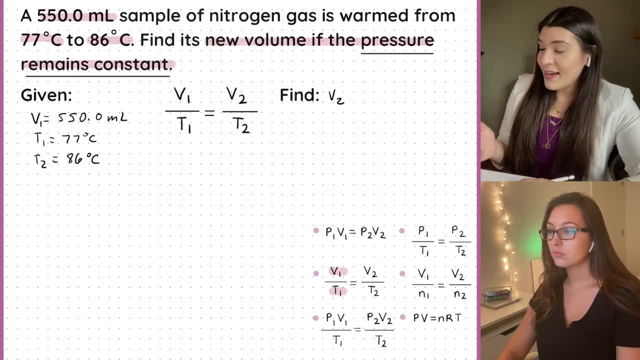 knowing which formula to use. Um, it's really just remembering them all. Perfect. So then the next thing we want to do, before we just start plugging everything in, is make sure that we do add 2.73.. This is a built in method And it's going to convert. 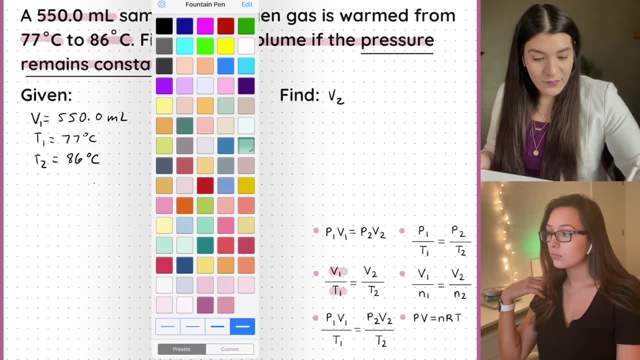 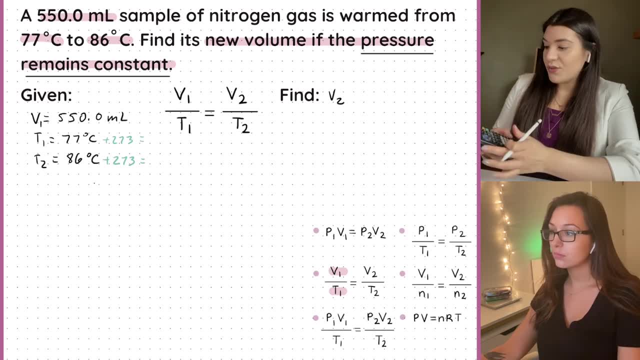 Well, 1, 3. zas, 42.3 degrees, That's going to convert both of these to KIlin. So if you were to plug it in and you wouldn't have converted anything, it would've been wrong. So let's just simply add: 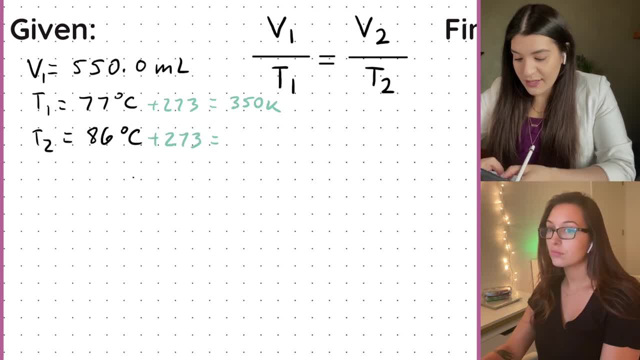 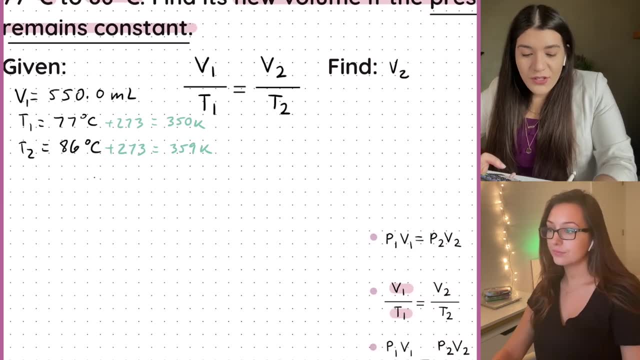 2, 73 to both of these temperatures and that's going to convert Celsius to kelvin, so I'll do that now be 359 Kelvin. Next thing, I don't have to do anything with these milliliters, I can just leave that. Just know that your final answer will be in milliliters. 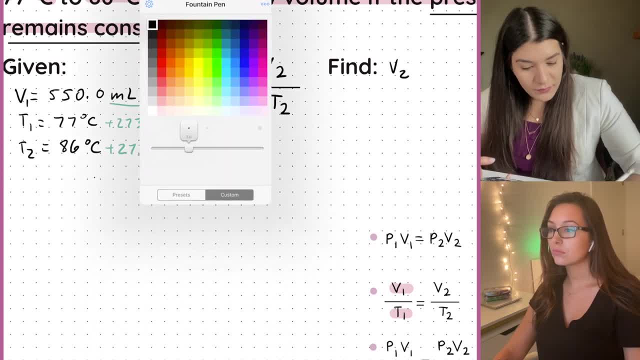 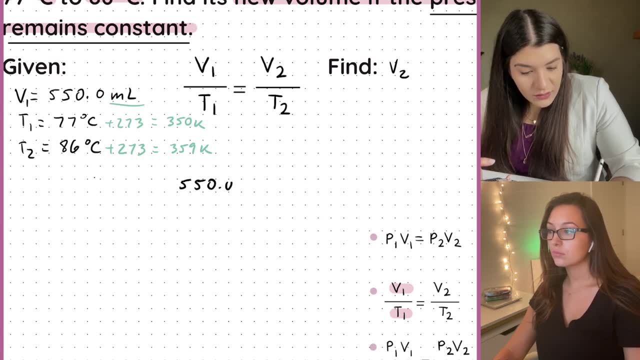 for volume. So I'm just going to plug everything in at this point. So on top I'll have V1. we said was 550, I'll just say milliliters for now, and then temperature: we just change this to 350 Kelvin. Next, V2 is what we're solving for. 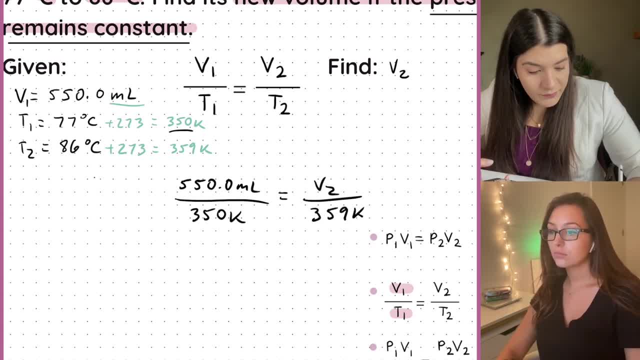 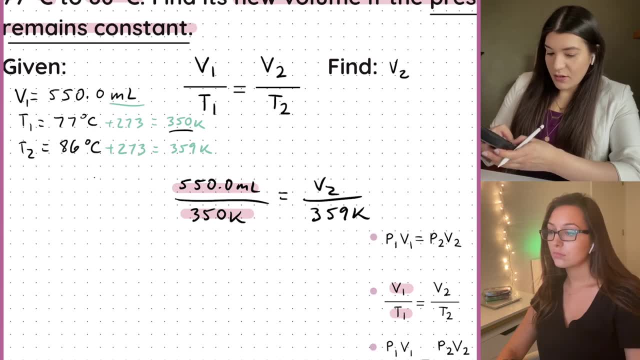 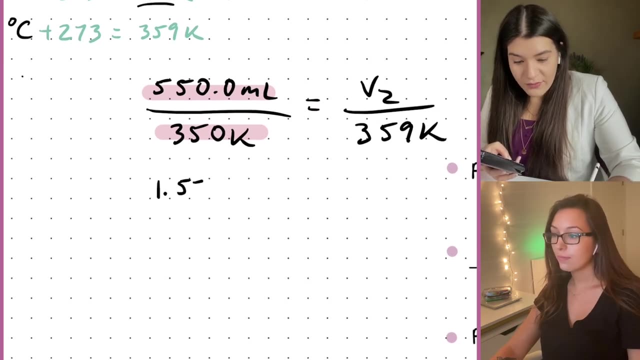 and then we've converted this one also to Kelvin. So what I'm going to start off doing is just dividing this, and then I'll handle everything else. So, just dividing these two values, we're going to get 1.57, and I'm not going to round at. 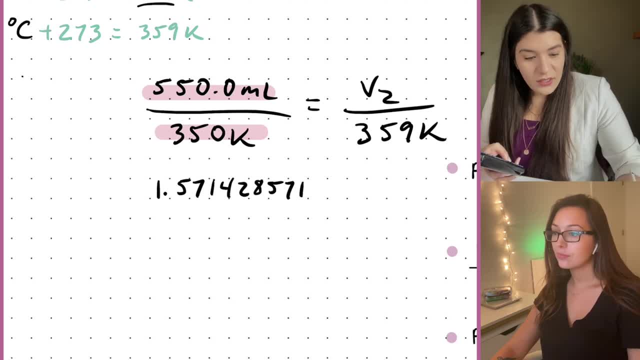 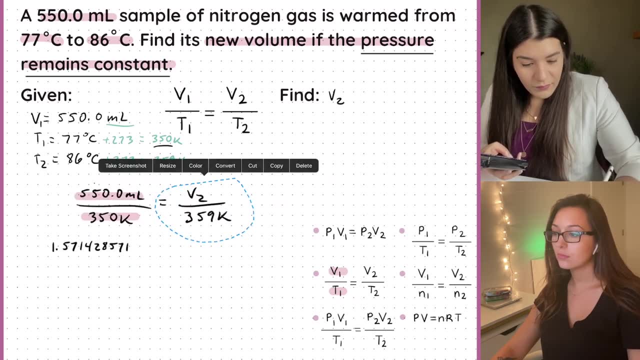 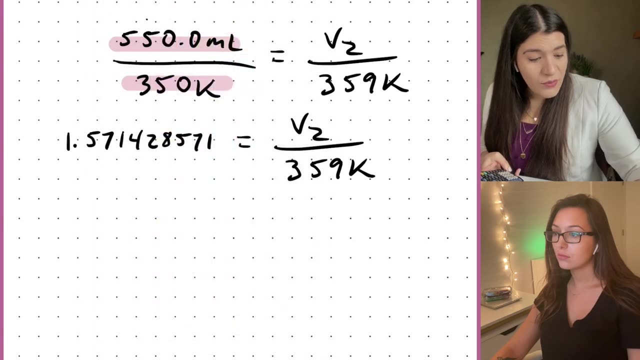 all I round, to the very end: 571.. Cool, let me move this over. Okay, next step is to simply get V2 by itself, So I'm going to remove this denominator by multiplying it by both sides. This would cancel, and I now have. 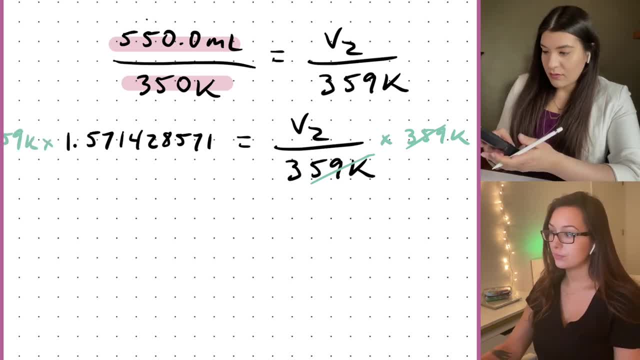 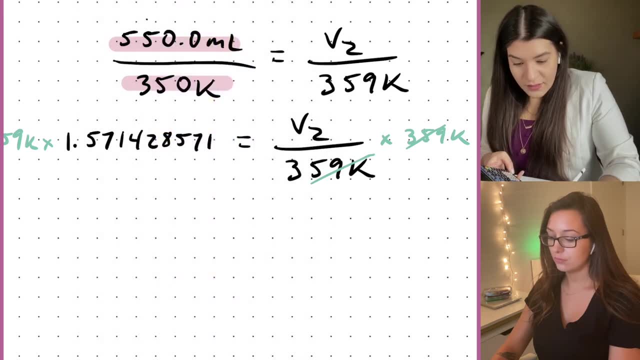 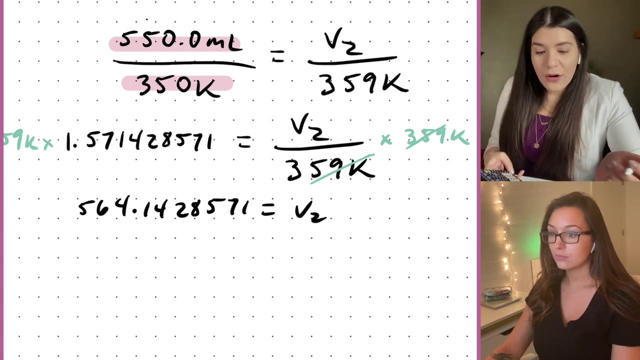 to multiply these two together, So times 359,, this is 564.14, then I'll round at the end. Just a little side note, as simple as that, to where the units go. this would have still have been milliliters divided by Kelvin, and then our. 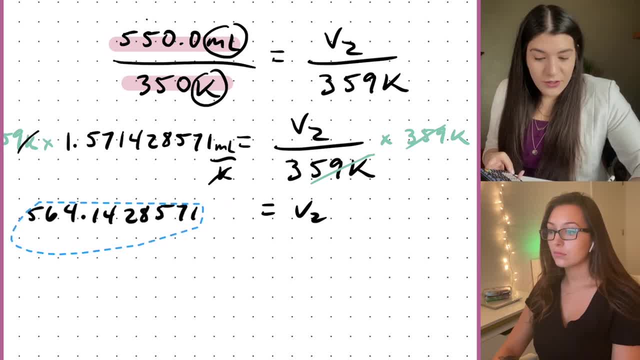 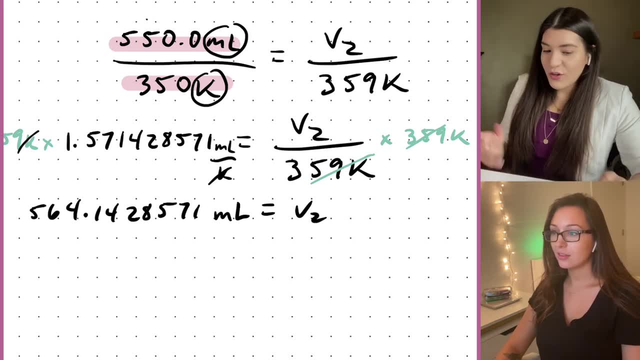 Kelvin and our Kelvin cancel, and that's why we're just left with milliliters. okay, I was kind of wondering, yeah, and then I mean plus, you could also just think of it as like the volume, it has to be in milliliters. it can't be in Kelvin or you know any sort of temperature unit. then our final: 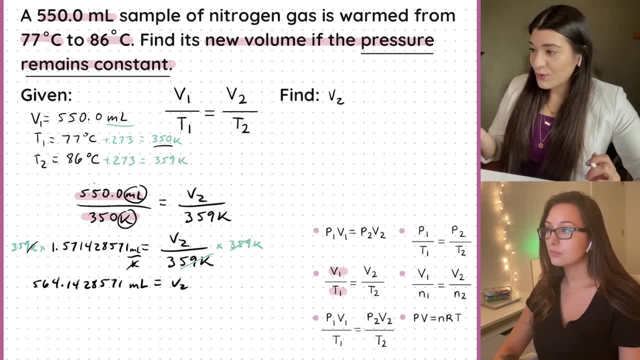 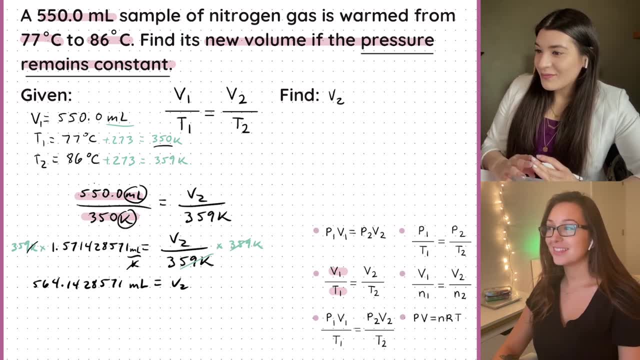 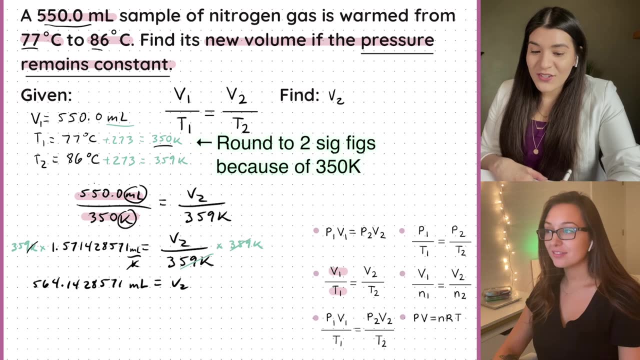 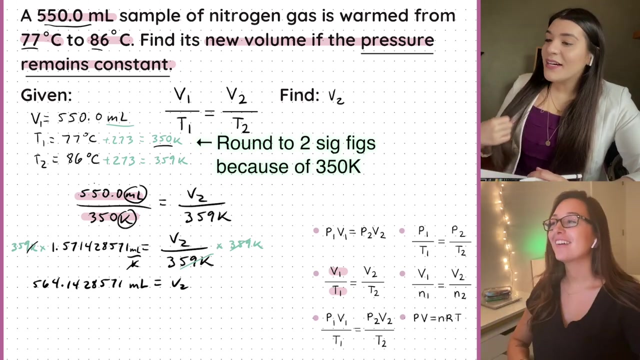 answer. so how many sig figs should we round two? um, oh, I think four, right, because they all count. so for this one, yes, but for temperature, there's only: oh, we're just looking at the temperature, so we're looking at everything. yes, yes, because it's division. yeah, but yeah, so it would have been. 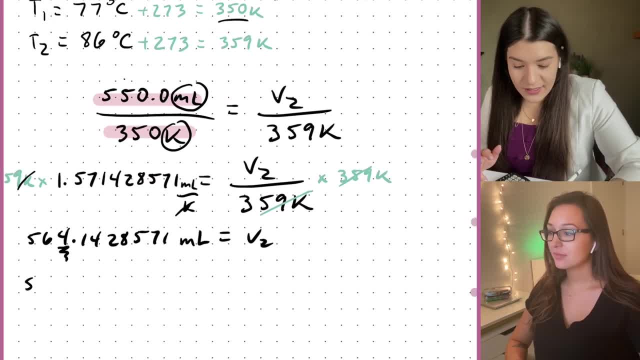 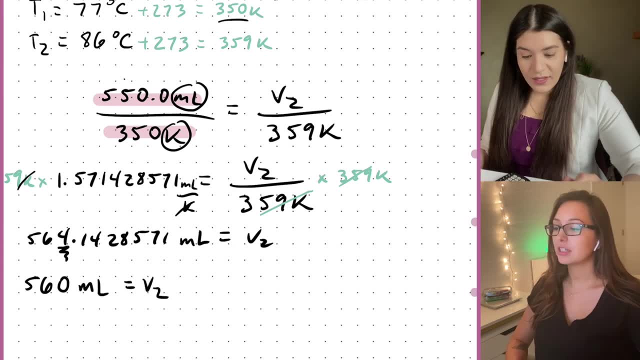 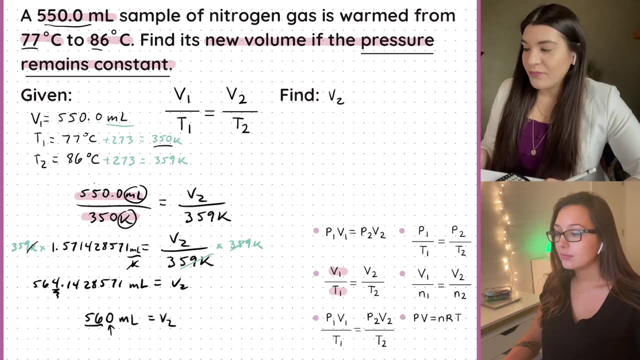 two. so I could actually round, round down you and say that this is 560 milliliters and that's our v2, that's our second volume, perfect, and that's it. cool, since we know that this zero does not count as significant, only these two count, right, cool, okay, moving on same sort of concept. so we're pretty much. 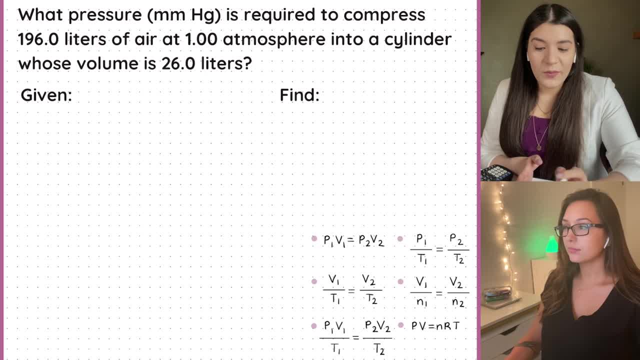 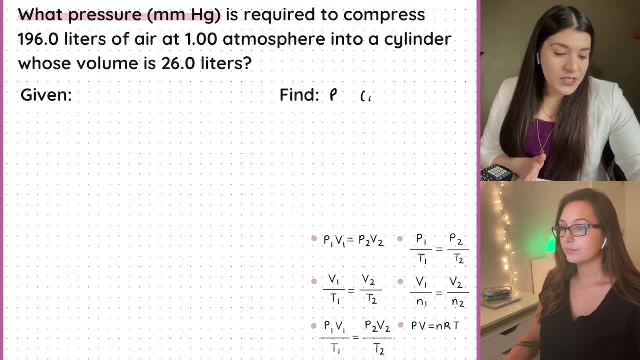 just changing the formulas, all right. so I'm going to start off and see that this is telling me what pressure in and it tells me what, like what unit it wants for pressure. so I know I'm looking for pressure and I specifically want this in millimeters. mercury, next, it's saying, is required. 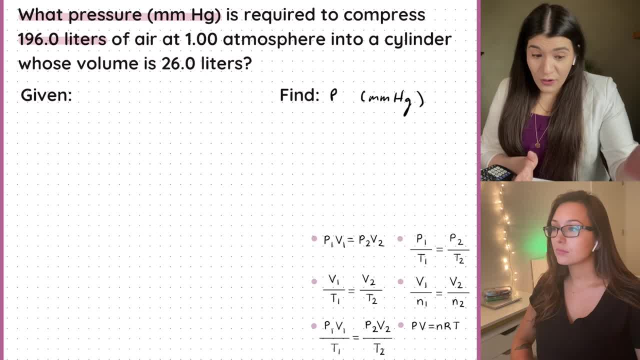 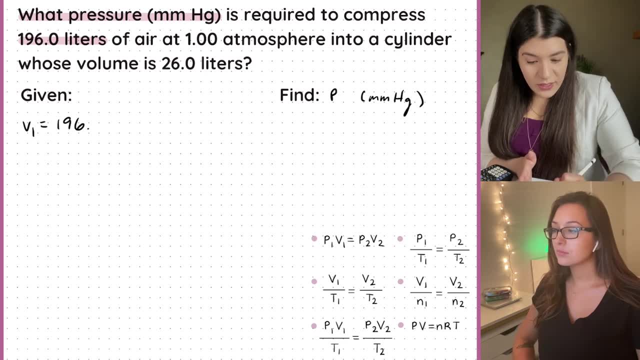 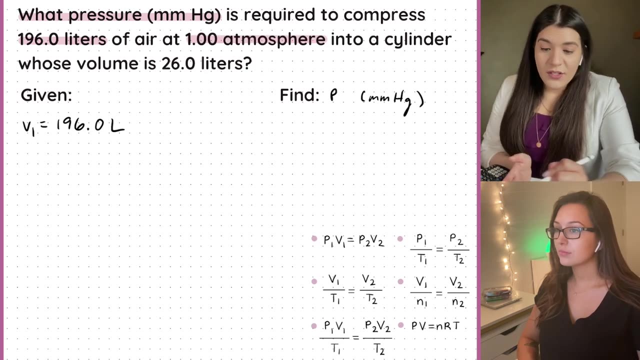 to compress this amount of volume. so I know liters is a type of volume, so that's v1, 196 liters and 0.0. and then of air at and then atmospheres is measured, is actually pressure. so I know atmospheres pressure. that's going to be my p1. 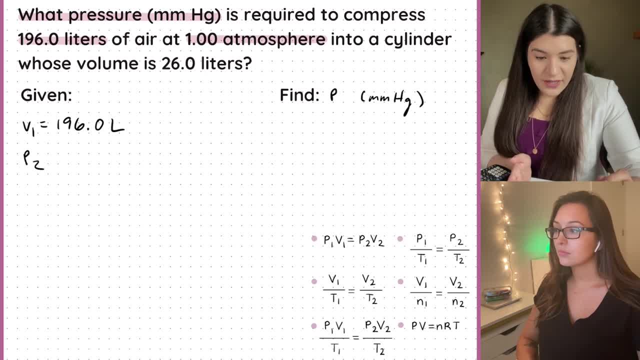 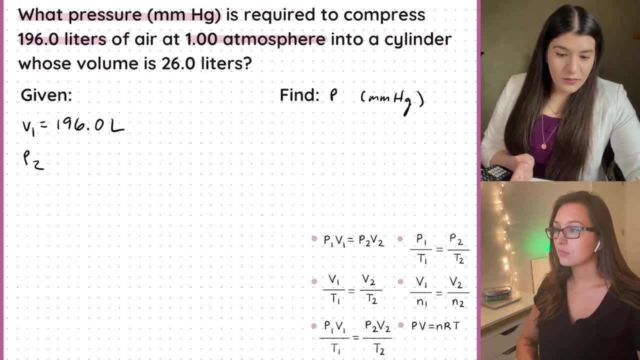 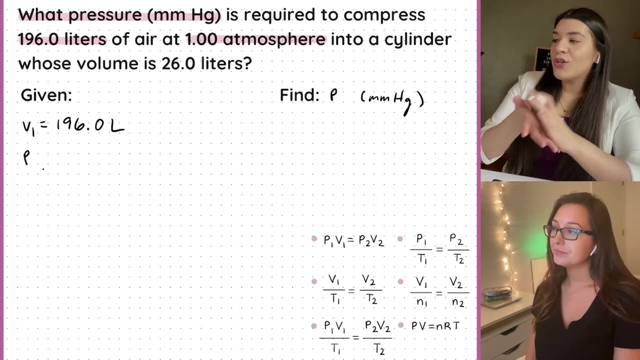 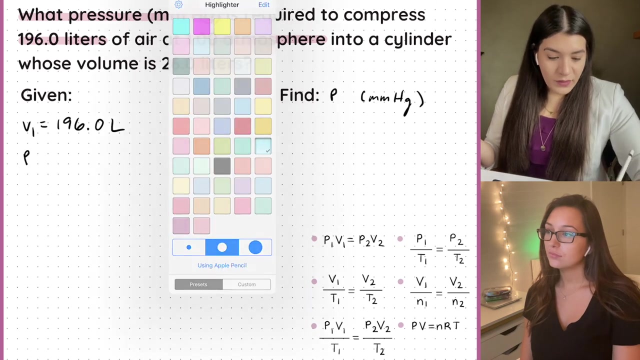 actually it's going to be my p2, and I'll explain how I knew that. um into a cylinder, whose temper, whose volume is that? actually it's not, and I'll explain why. so, um, the reason, like this is also important to know, like whether it's v1, you know p1, so on, um, how I can just tell, is this keyword of right I know. 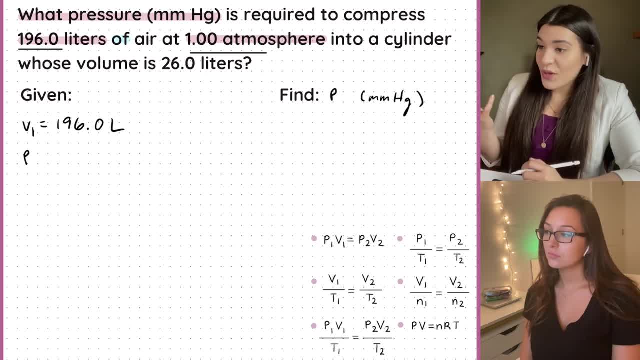 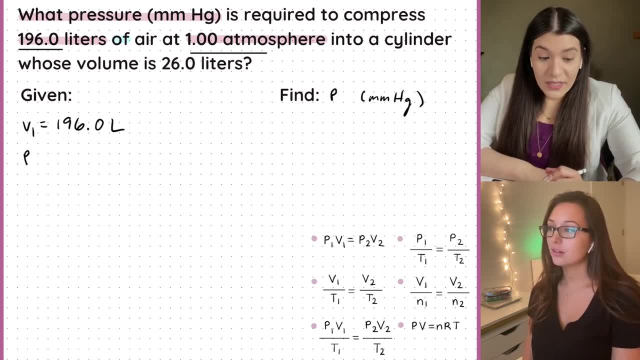 that these two have to go together. so I know that these two have to go together. so I know that these two have to go together, so those both have to either be one and one or two and two. oh, okay, okay, so it's p1 then. then it's p1, correct, okay? so that's 196, actually pressure, one atmosphere. 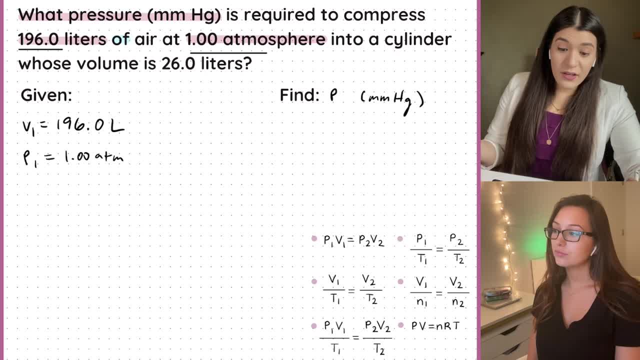 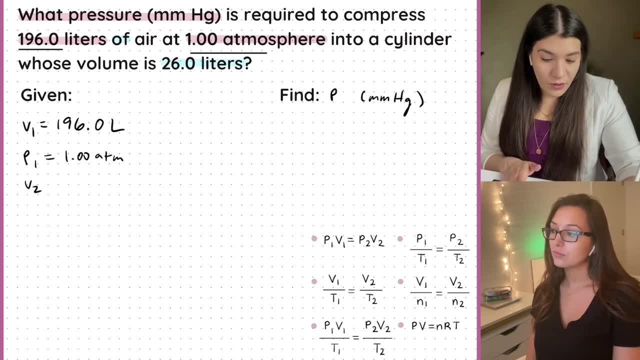 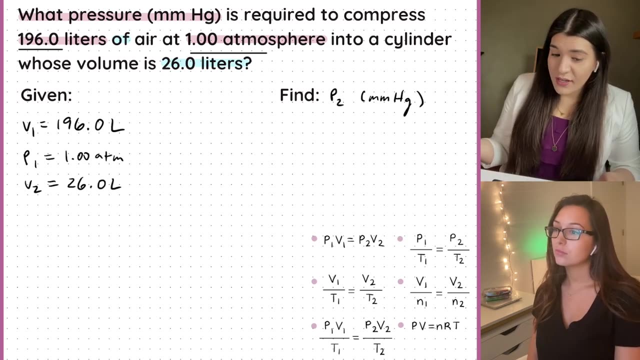 point zero, zero atmospheres, yeah, and then next they're giving us a second volume. so I know that this is going to be my v2 and I'm looking for p2, and then, luckily, I don't have any temperature, so I don't have to convert anything. 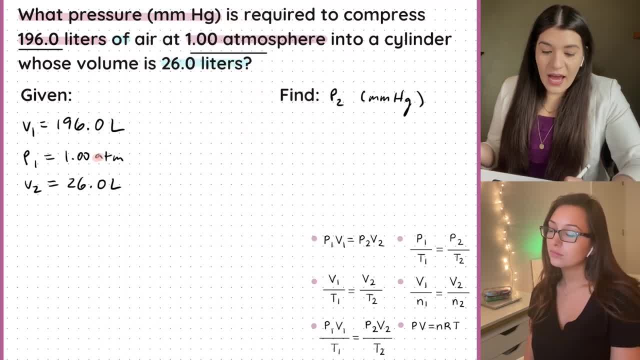 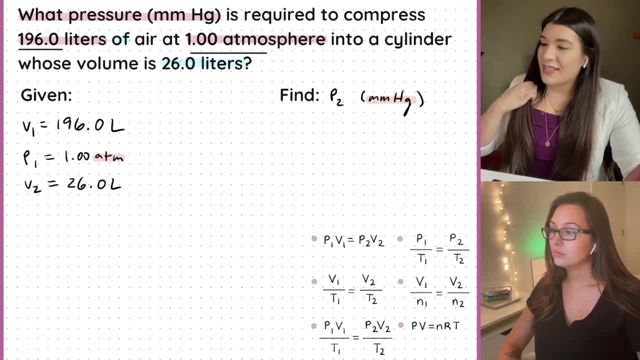 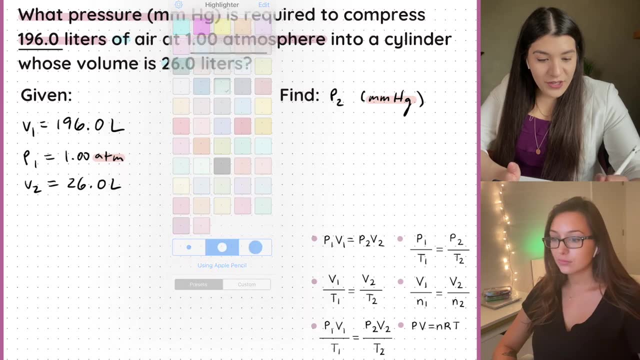 next? I could either decide to convert this atmospheres to millimeters mercury right now, or I can do that at the end. really doesn't matter, it's not going to change the answer. I'm going to do it at the end just to make it easier. so first I have to figure out what's the 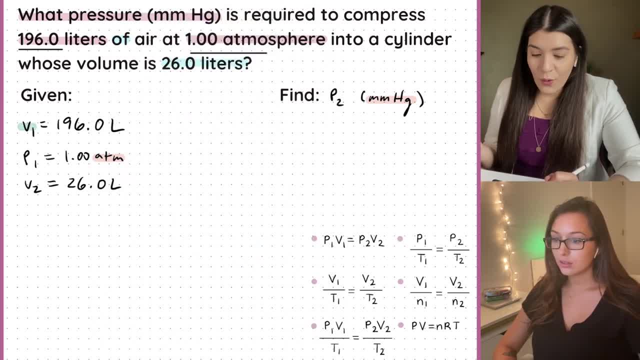 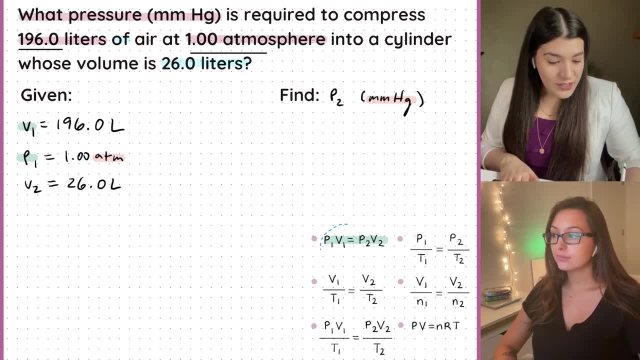 formula. so what's the formula that is going to, you know, only have volume and pressure. well, it's the as one right, only volume and pressure. that's all I'm worried about. so I know that I'm using this, and if you were given all of them, that would be so easy, right? yeah, I wish. and then, from here, I 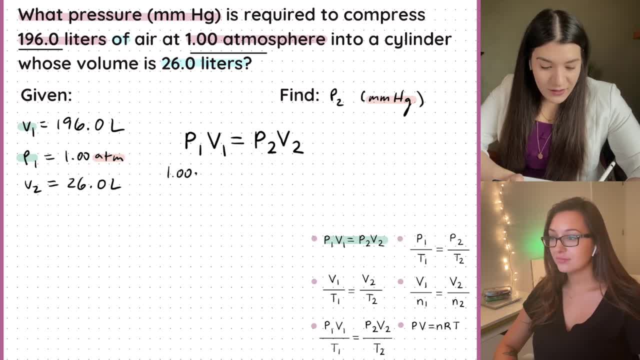 just plug everything in. so I know that p1, we said, was one atmosphere, b1 was 196 liters- is equal to b2, which is what we're solving for. the last condition is that, basically, if I do that rightل for and v2 is 26.01 actually 0 liters, next i'm simply going to- i'm actually going to do this. 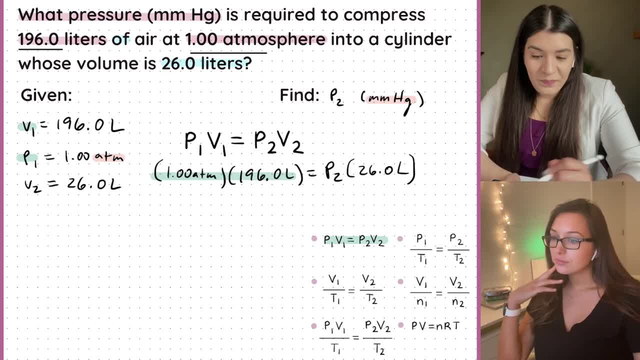 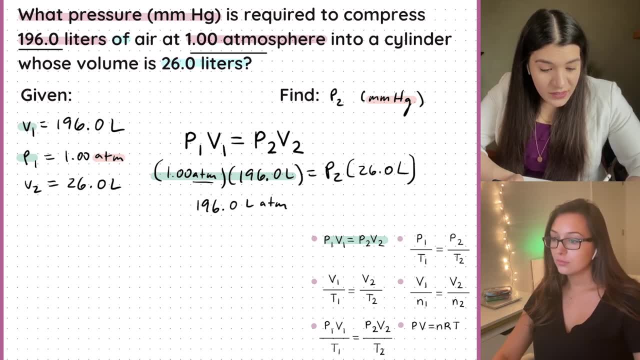 on. actually, i can just really just multiply that. i know it's just the same thing, right? 1 times 196 is just going to give us 196.0, and i'll say this is liters times atmospheres, since these two combine. and then next all i have to do is divide that 26 liters to both sides to find my answer. 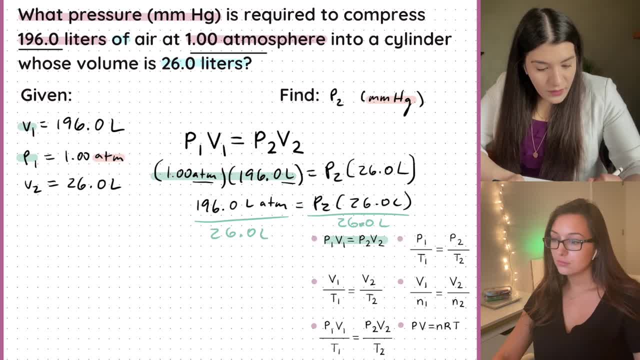 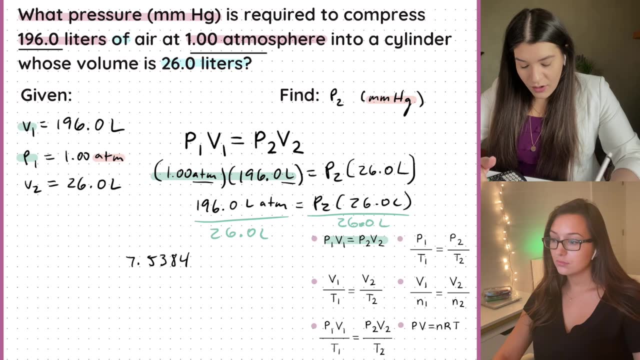 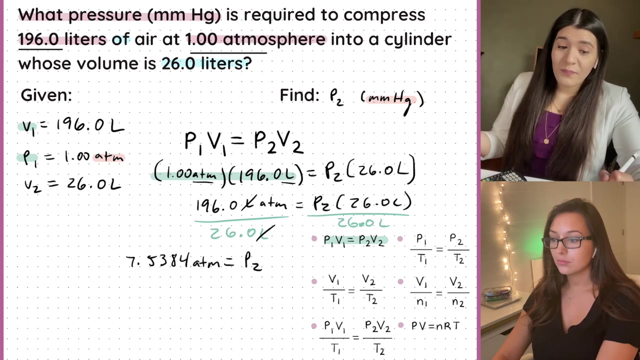 what would that be okay, and let's see what that gives us. so 196 divided by 26 p2 is equal to 7.5384 um. and then remember that liters and liters would cancel, leaving us with atmospheres. and this is p2. but we're not done yet. we wanted our final answer to be in millimeters. 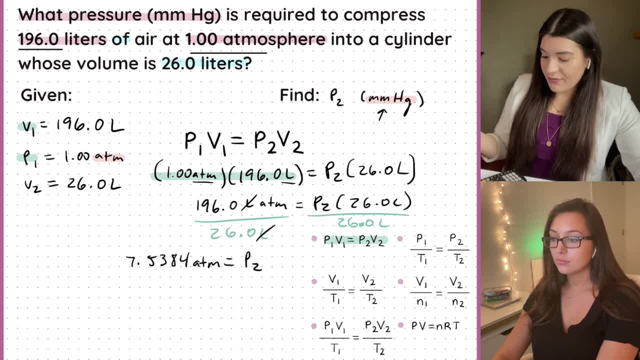 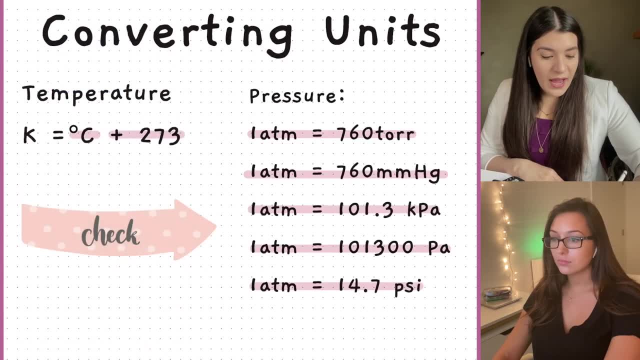 mercury. so i'm going to convert this and then i'll de-estimate it. okay, so this is what we want to do with this. so we want to convert this. so we're going to go ahead and convert those to a minimum with sig figs and all that. so this goes back to our unit portion of this, where um one atmosphere. 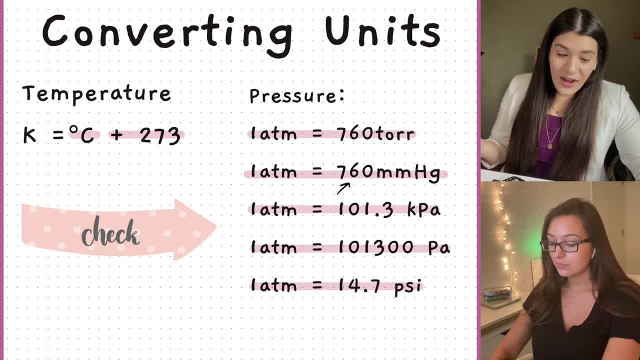 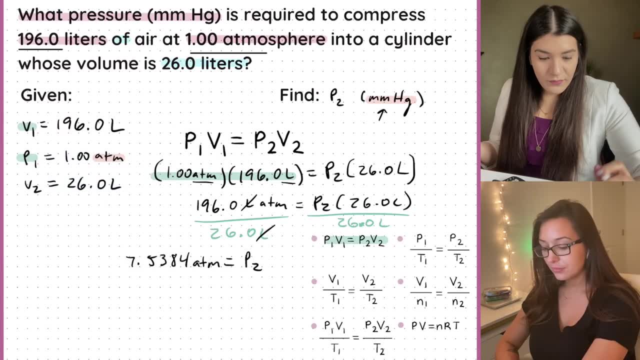 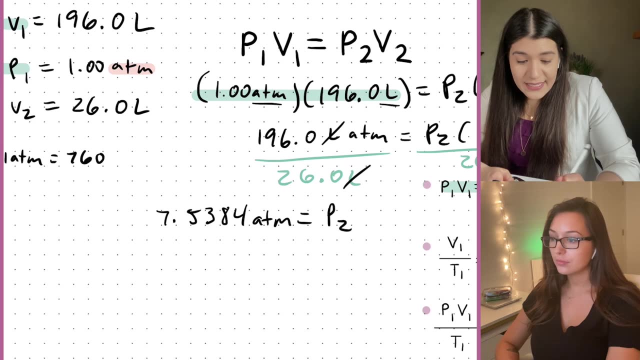 is equal to 760 millimeters mercury. so i that's something that you just had to remember, okay? so i'm gonna actually do this and just show that. that's where i took it from. i know that one atmosphere is equal to 760 millimeters mercury. that is my conversion factor and i'll convert this. 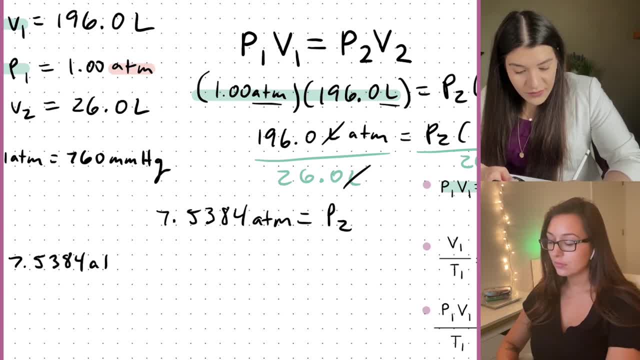 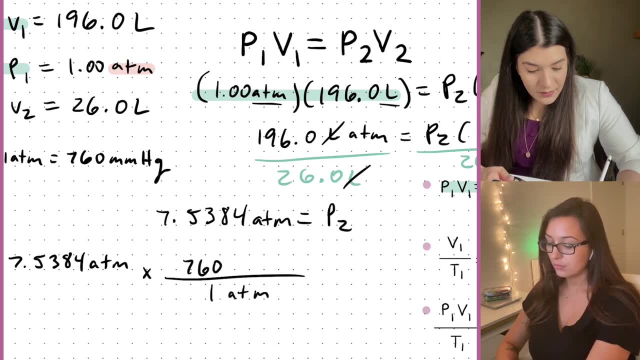 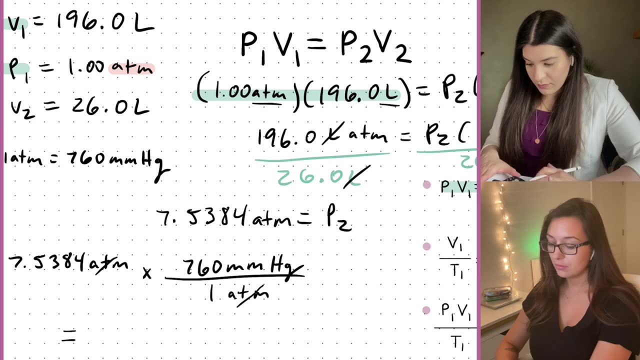 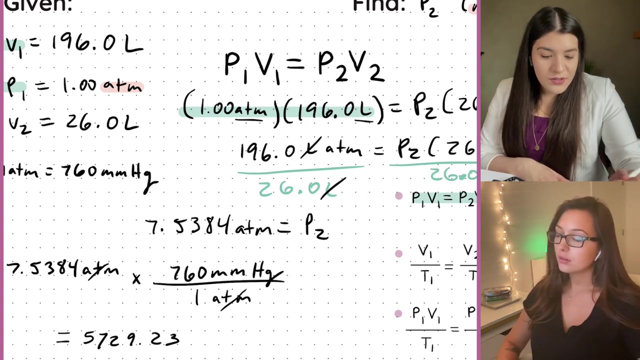 so 7.5384 atmospheres. multiply this by one atmosphere on the bottom and 760 millimeters mercury on top. atmospheres, atmospheres cancel, and let's see what that gives us. so this would give us a five, seven, two, nine. point two, three. just a little side note. i didn't round. 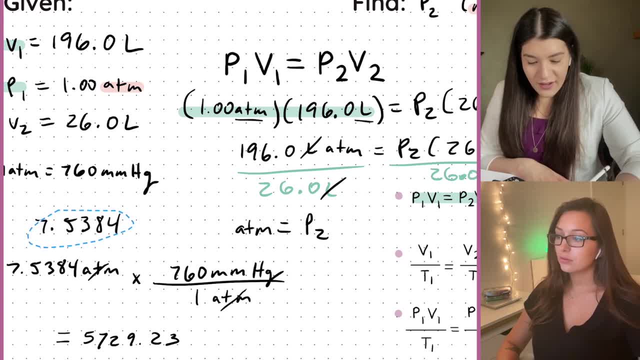 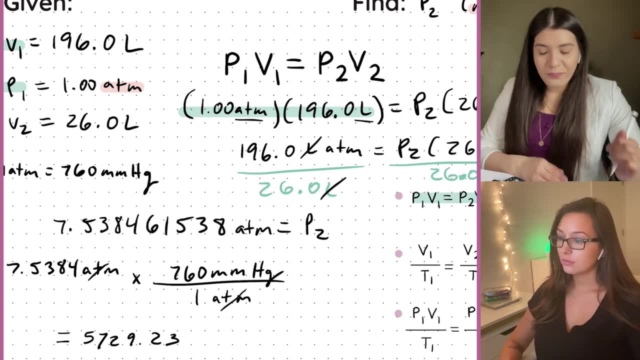 this part, like i'll actually write everything out that i, that i put i had in my calculator. this was six, one, five, three, eight. i don't want to round until the very, very end, so that's what i actually put here. so perfect. and the next. this is millimeters, mercury. 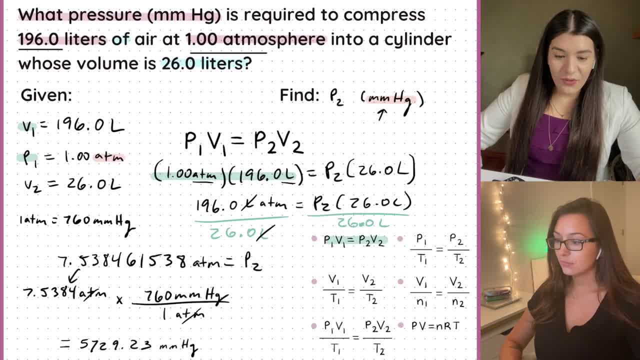 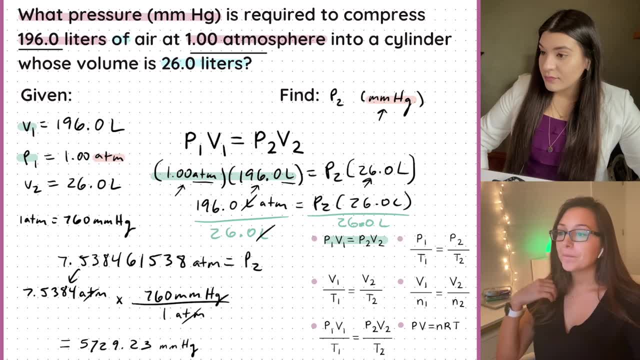 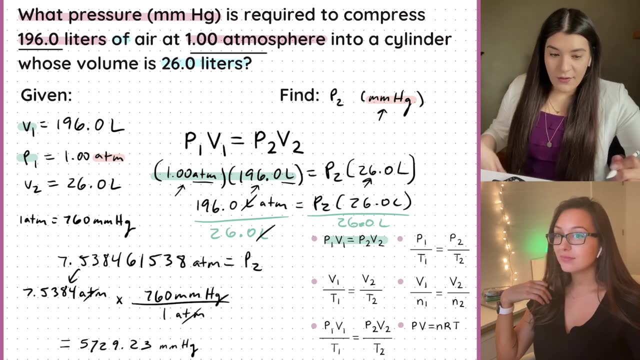 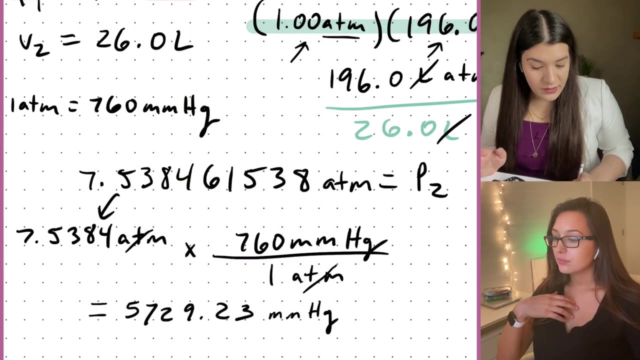 last step is just to figure out our sig figs. so, looking back, since everything is multiplied, what's our least amount of sig figs? um three, yes, so i have to round to three sig figs. so, that being said, we're gonna actually round up. so, if we see here, we only want three sig figs, so i wouldn't just say 572, because that's different. 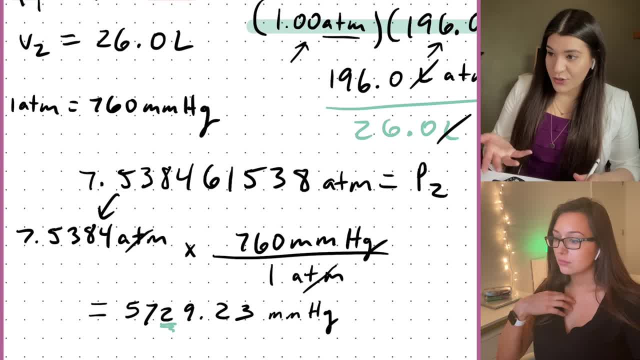 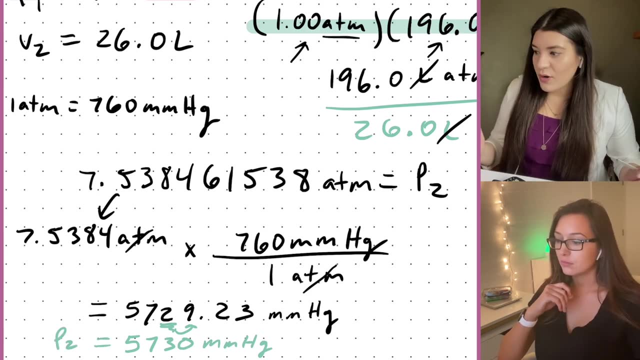 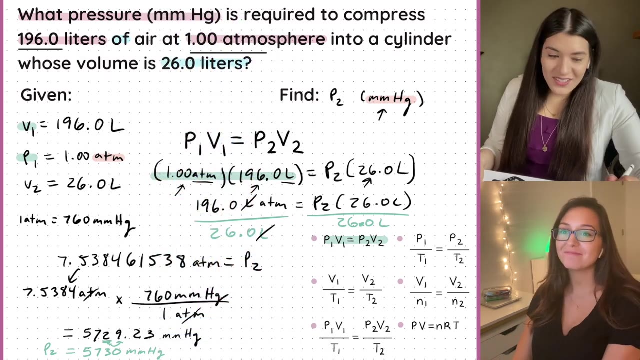 that changes the number entirely right from 5729. so i would just round this up to 30.. so i look at this next, next number and i say, okay, three's next. so this would be my answer. so this was p2 questions here. no, no, that's not bad, just need to learn all of those. yes, that, that's really it. uh, perfect then. 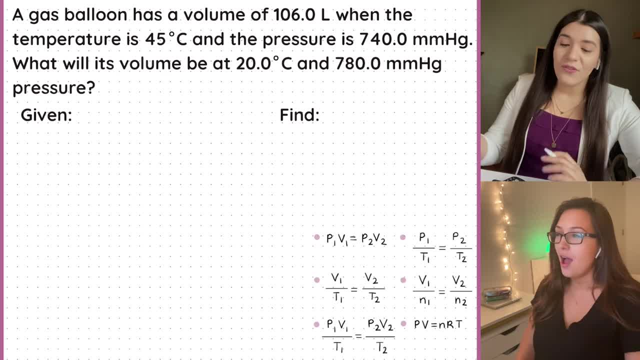 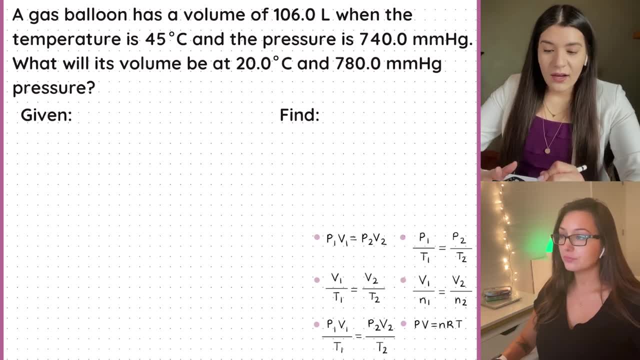 the next one. so still the same sort of concept. i'm still going to start off with what's my given, what's my finding, and then figure out the formula from. you know what's given and what i'm finding. so it's saying a gas balloon has a volume. so right there. okay, i know i have volume, so i'm. 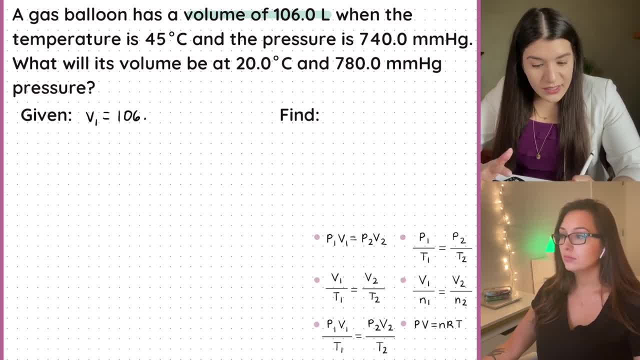 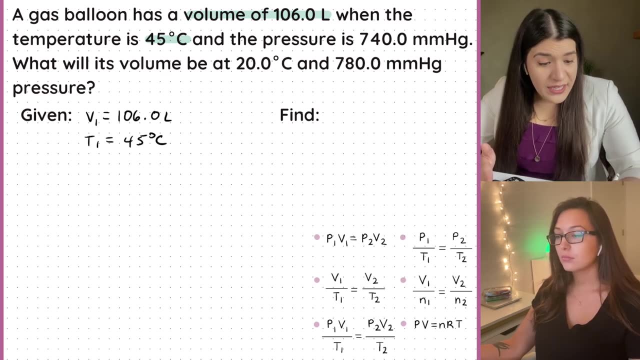 going to say i have v1 is equal to 106.0 liters. next, uh, that amount when the temperature is so okay, i've got a new temperature, so t1, 45 degrees celsius next, i see, and the pressure is so pressure, it's this one's kind of nice. 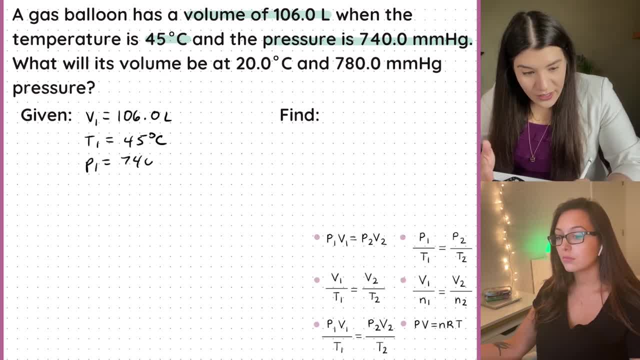 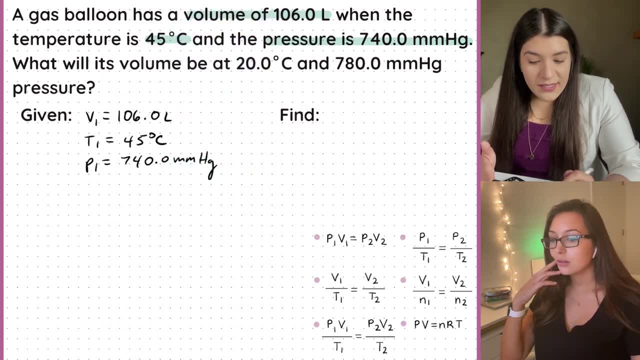 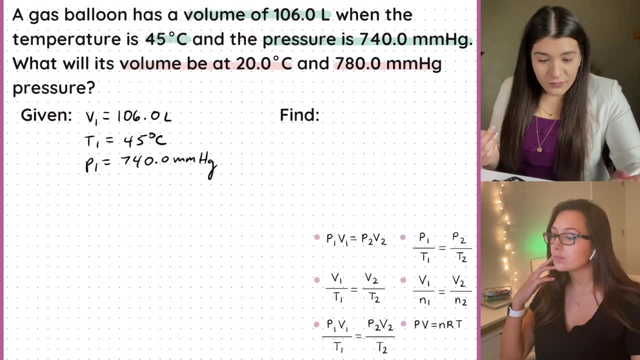 literally tell me, telling me what everything is. so, 740.0 millimeters mercury, and it's asking: what is, what will its volume be at? and now it gives me a new temperature, a new pressure. so i'm going to say so. i know this is going to be a larger formula, since i'm asked to find, you know, what's the new. 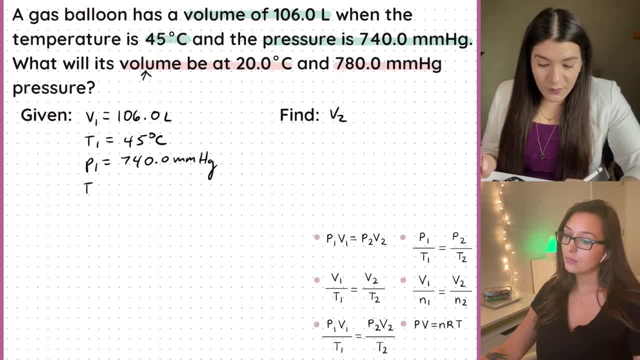 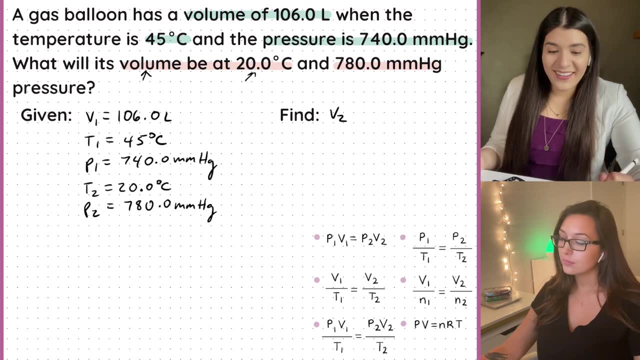 volume. i'm going to solve for v2. they also give me another temperature here, so t2 is 20 degrees celsius and then a new pressure, so p2 is 780.0 millimeters mercury. so since i have basically kind of like duplicates of everything, right, i have two v uh volumes, two temperatures, two pressures. i 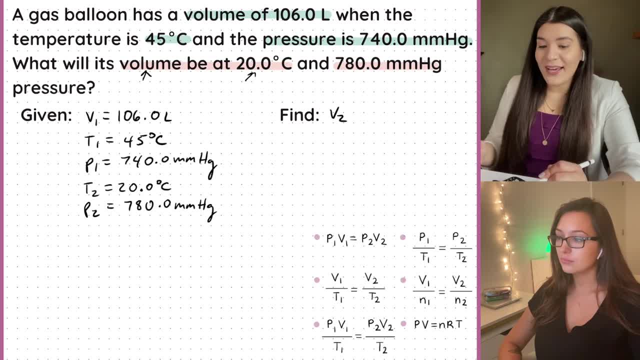 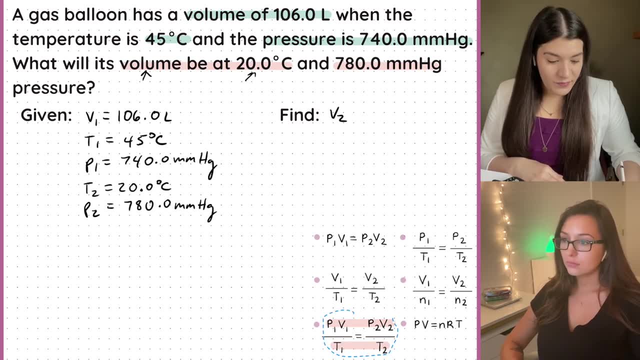 know that the only one that combines all of these is the combined gas law, which is this right, it has everything. so that's the formula i'm going to use. so it's gas laws. i think it's just. yeah, it's really just remembering all the formulas and knowing what to plug in where. 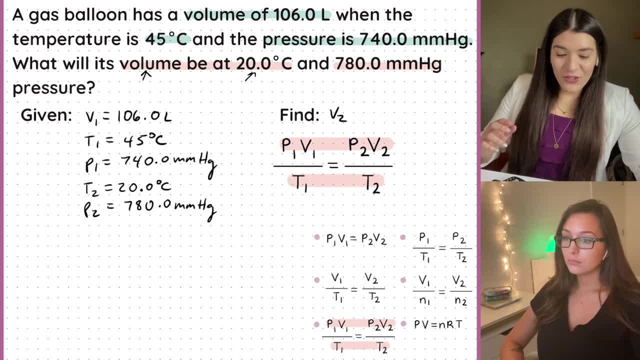 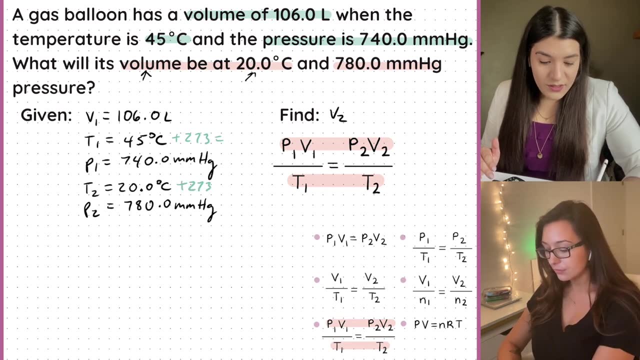 but other than that it's not too bad. and also knowing to convert your units. so units here: the only thing we have to convert is the temperature, right? if there is temperature, you always have to change it to kelvin. so i'm simply going to add 273 to both temperatures so i can convert this. 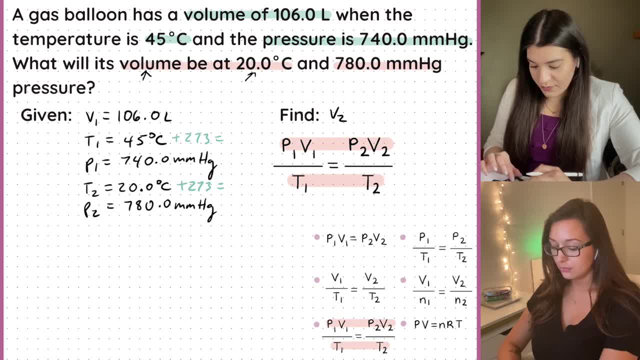 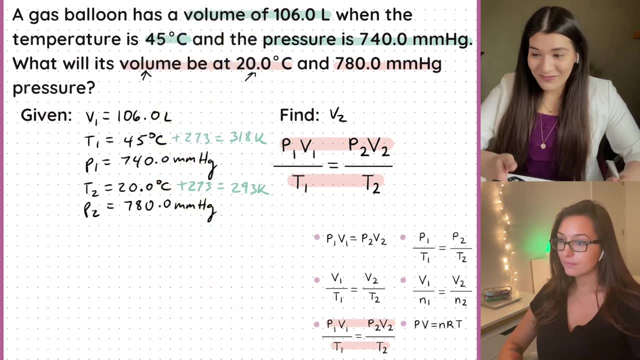 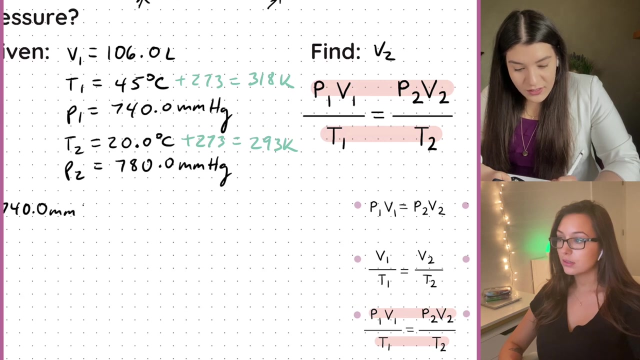 so let's see what that gives us at 273 plus 45, to give us 318 kelvin, and then 20 plus well, 273, that's going to be 293 kelvin. perfect, and next thing is really just plug everything in. yeah, cool. so i'm going to start off with the first pressure. it's fine that it's as long as these. 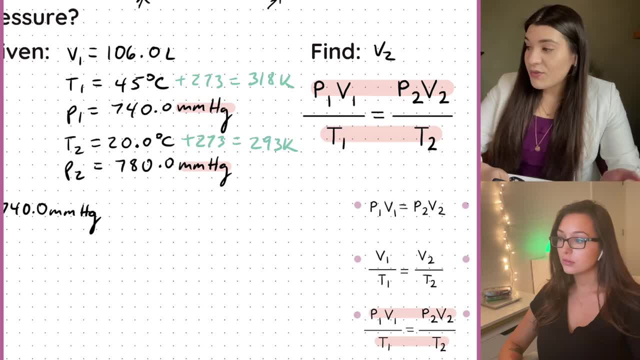 two little note. as long as these two are the same unit, you don't have to convert anything. but if this was in, let's say, atmospheres, then you would have to convert either you know this one to atmosphere, like both of these top and fear atmospheres, or both of them to millimeters mercury. 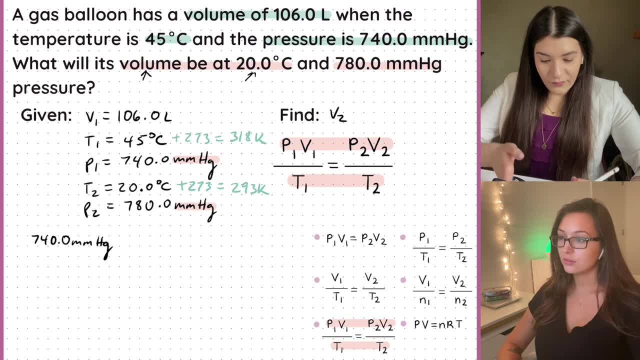 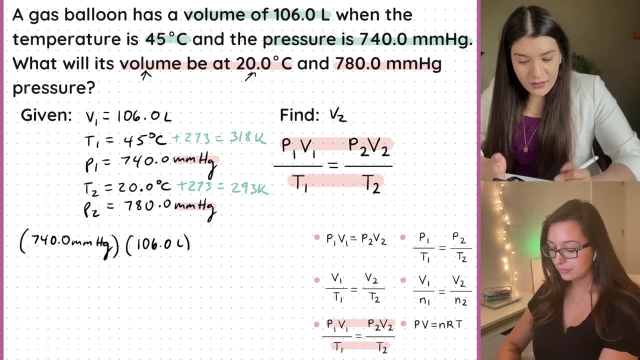 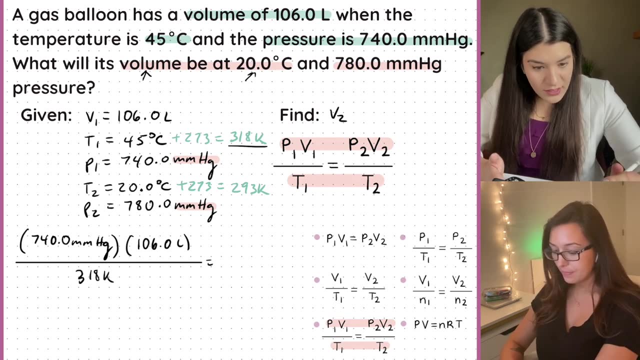 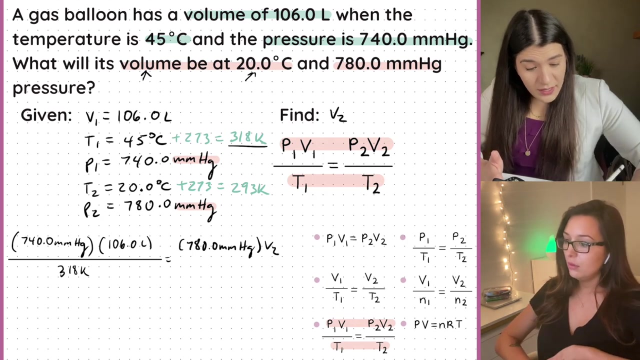 they just have to be the same. good to know, cool. so v1 was 106.0 liters. then city t1 was our new value of 318 kelvin and i'll set this equal. i need more room to p2, which was a 780.0 millimeters mercury. v2 is what we're solving for and then t2. 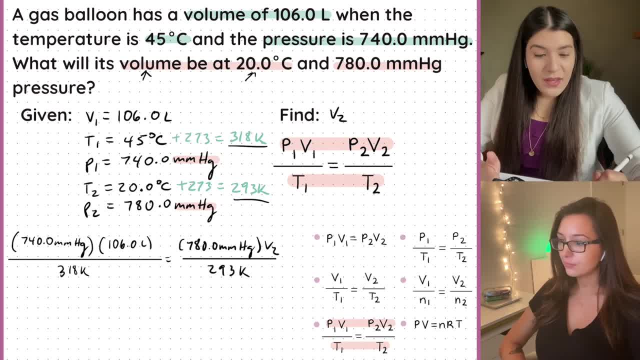 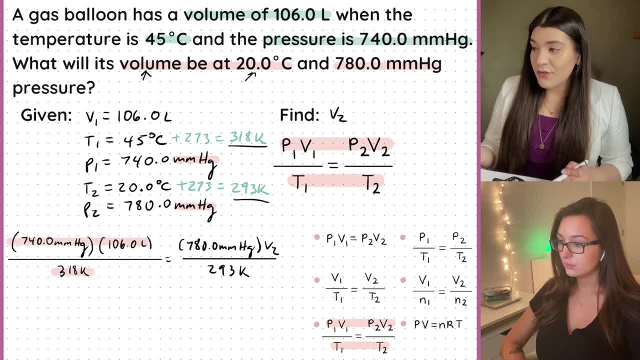 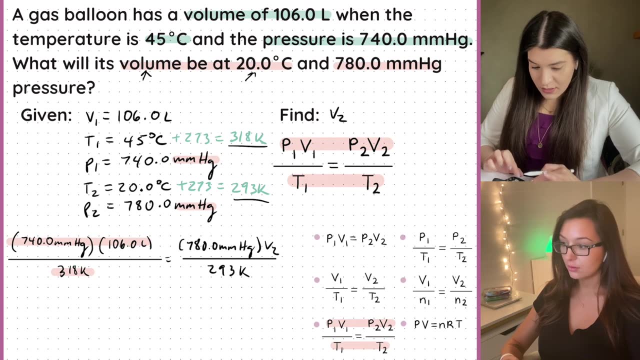 is 293 kelvin. okay, so let's just start off with doing all the math. what i'm going to start off with is the left side, so i'm going to multiply these two together and then i'll divide by 318.. so 7, 40 times 106. so i'll just write what it actually gives me. so that gives me seven eight. 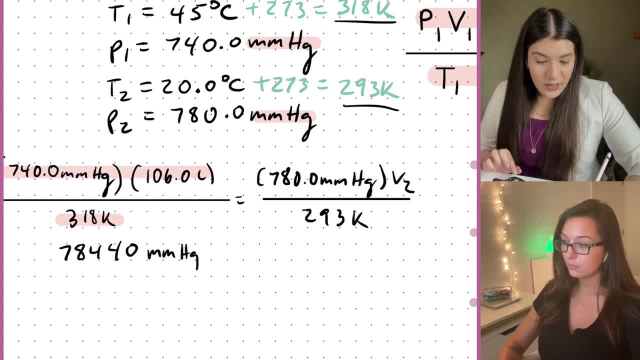 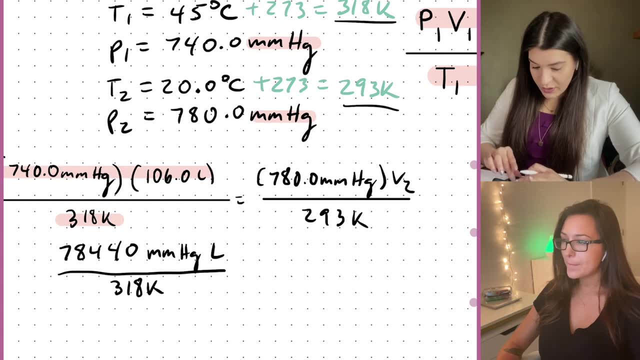 four, four zero. i'm gonna say this is millimeters, mercury times liters, and then this is still divided by 318 kelvin. so now i'm going to do this next part, so i'm going to divide those two values. so i'm going to do this next part, so i'm going to divide those two values. 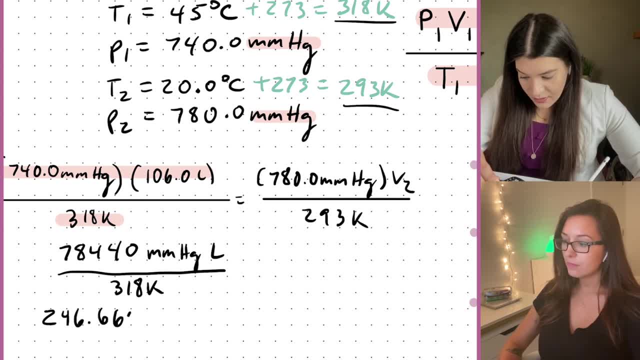 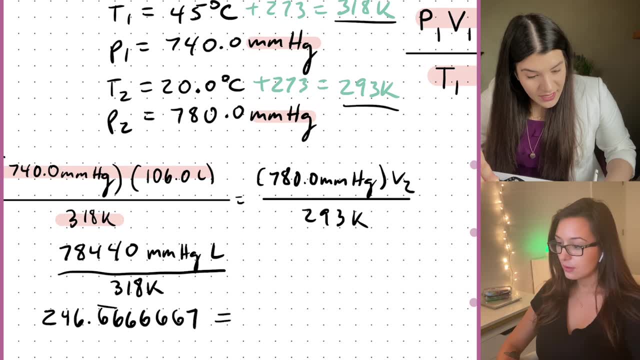 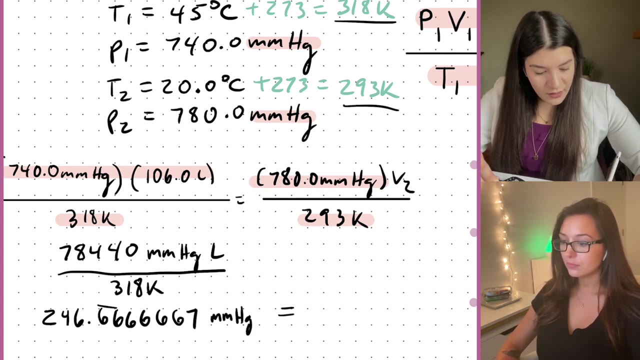 so 246.. a lot of sixes, um, and i'll say seven to seven. there we go. this just repeats. so the next. i'm going to now divide these two values, just to make our lives easier. so this is you know what. let me put the units as well. this is still millimeters, mercury times, liters, divided by. 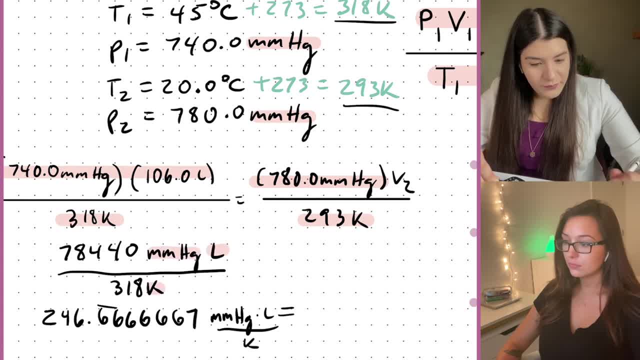 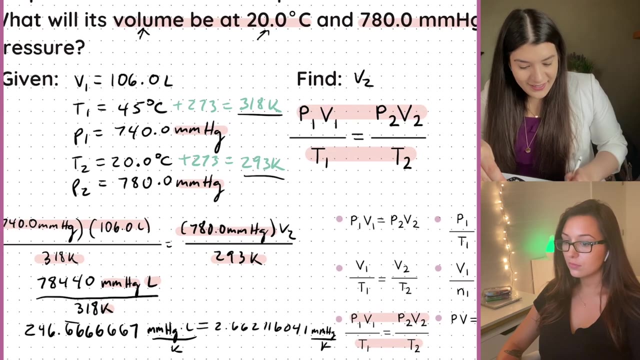 kelvin. since that's where i get it from, i'll divide those two values. so 780 divided by 293, that gives us 2.662116041, and this is millimeters mercury divided by uh kelvin. okay, give me a second, probably going to remove some of this stuff just to make our lives easier. 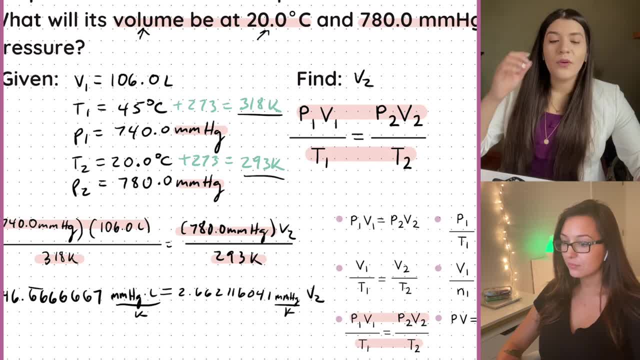 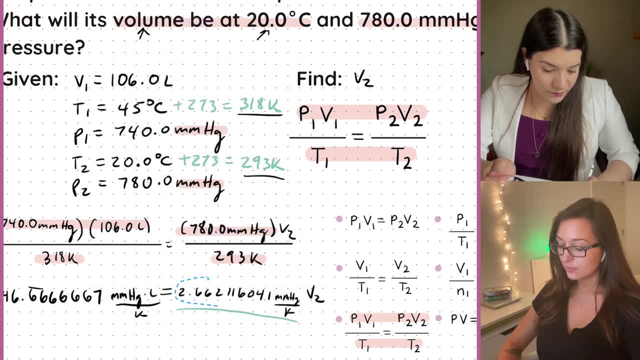 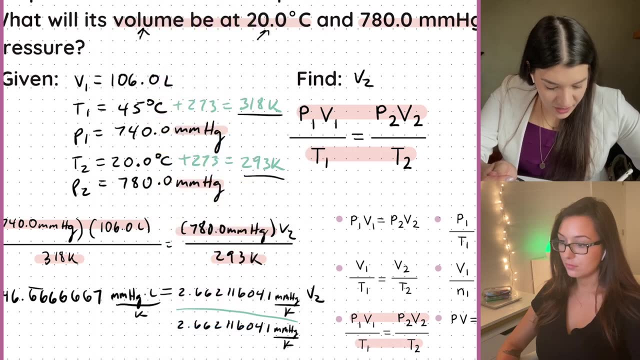 okay, and i still have v2 here, since that's what we're solving for. next step is to simply just divide. so that's what i'll do. i'll divide this whole entire thing over, so nothing too tricky here. i'd say it's pretty straightforward, just knowing what formula to use. 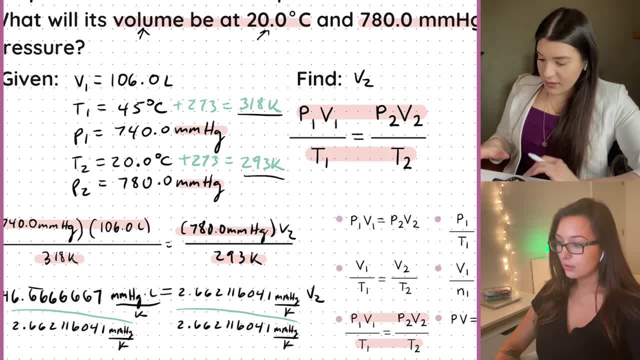 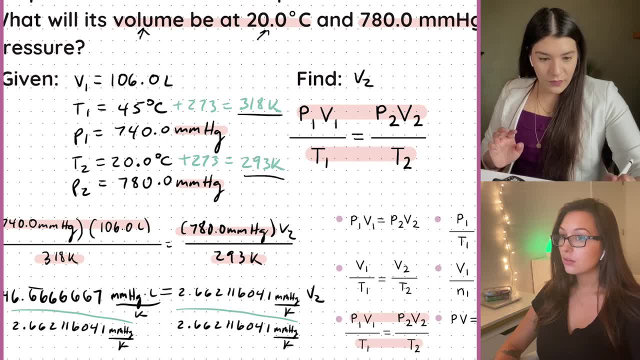 yeah, cool. so let me divide that and see what we get. so two, four, six, that whole number, um, okay, so i get, and i'm just going to put it up here- i get v2 is 92.658 and then i'm going to see how many sig figs we need to round to. so just looking at, i'm going. 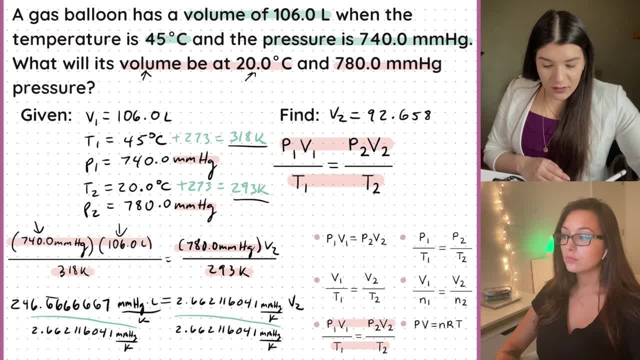 to actually look at everything that we multiplied here. so just seeing what is the smallest amount, well, the smallest amount would have been the kelvin right. so three sig figs would be our final answer. so i'm going to round up looking at that: five this would have been: 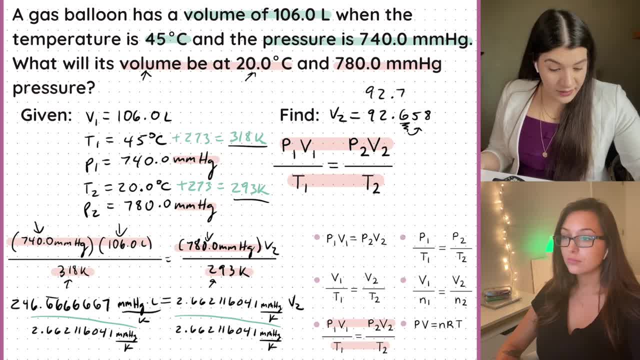 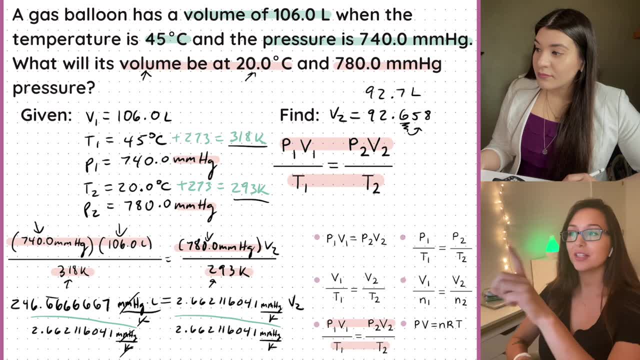 um Первz Тут Life. dot 92, .7 um, and this would have been uh, liters. okay. so in this instance it was okay to be in liters, because it gave it the initial one in liters, correct, and they didn't specify. so if they would ask like: oh, i want like, like what? 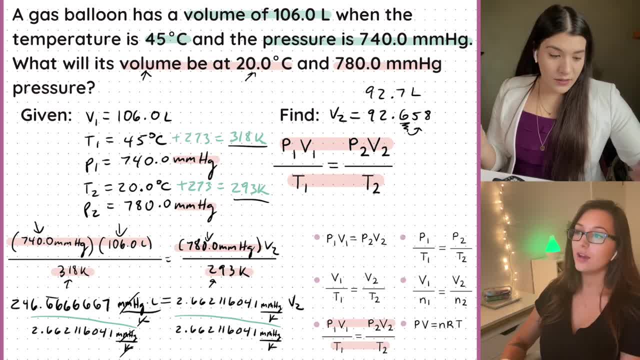 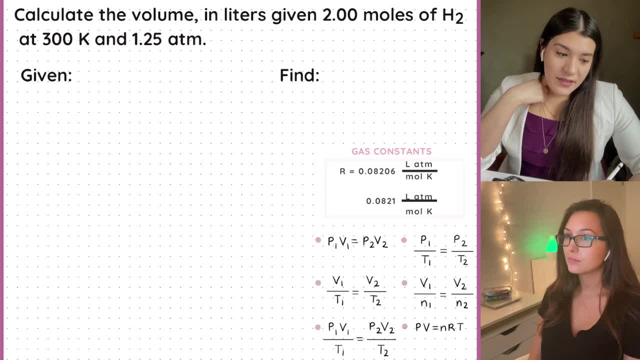 is the volume in milliliters, then we would have had to convert it after: okay, cool, perfect, uh, all right, so this one's a tiny bit different. um, i would say that this is a different formula, and that's kind of why theре will be larger. 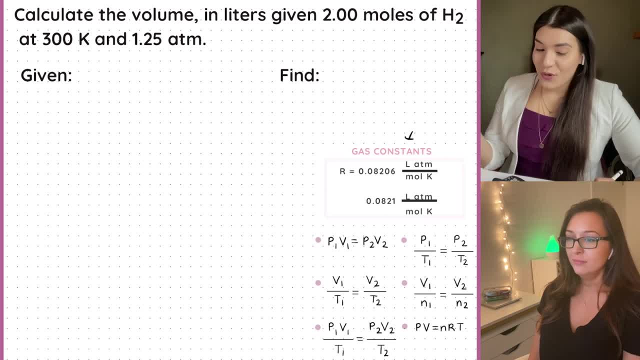 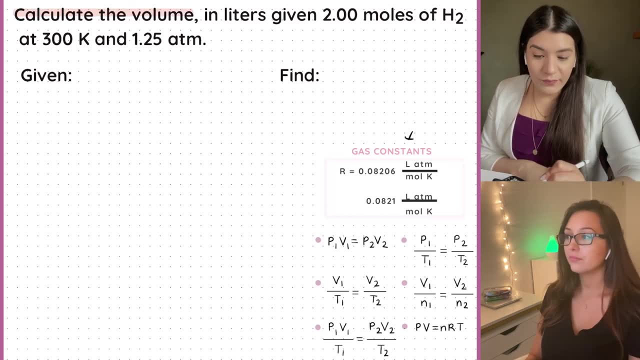 kind of why I have these gas constants. But I'll explain how this works. So, once again, what's given? What are we finding? Well, we're asked to calculate the volume, So our volume. Next, they're giving us in liters. So actually, this tells us right, This tells us. 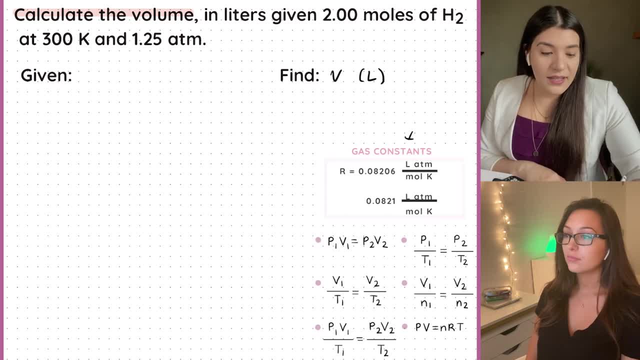 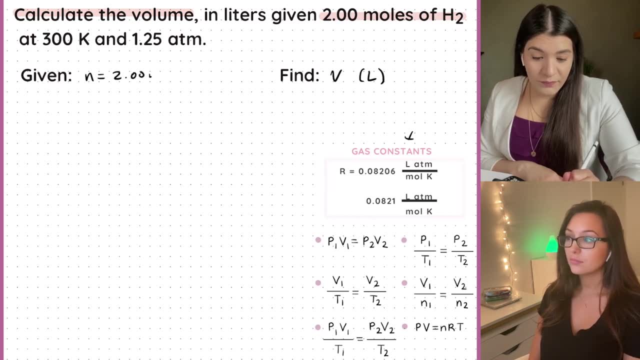 that it wants the volume in liters. Next it says: given two moles of H2.. So now I'm giving moles, So I know N is two moles. Next it's telling me the temperature. Luckily that's already in Kelvin. 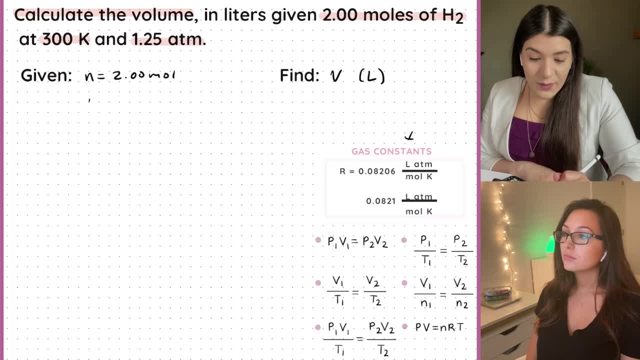 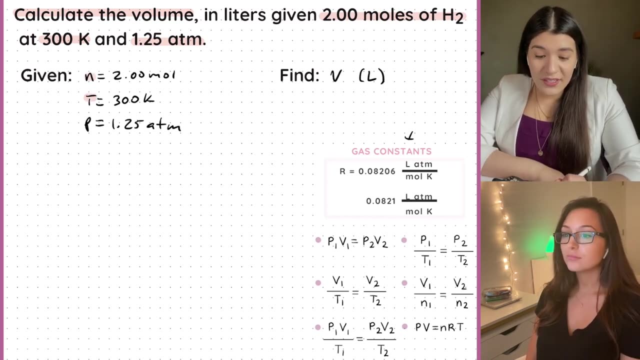 So our temperature and our pressure. So we're given temperature 300 Kelvin, and then we're also given pressure, So 1.25 atmospheres. Okay, well, what's the only one that allows us to, you know, basically combine everything and it's not like duplicates of them, meaning. 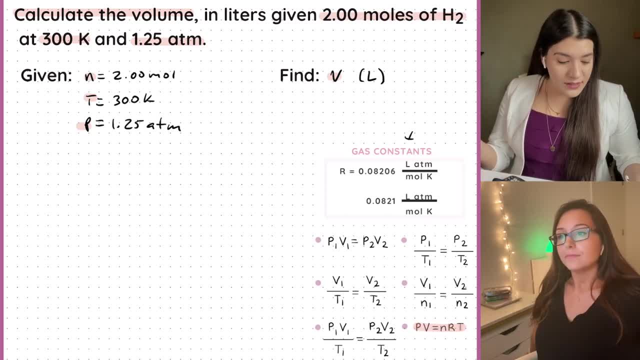 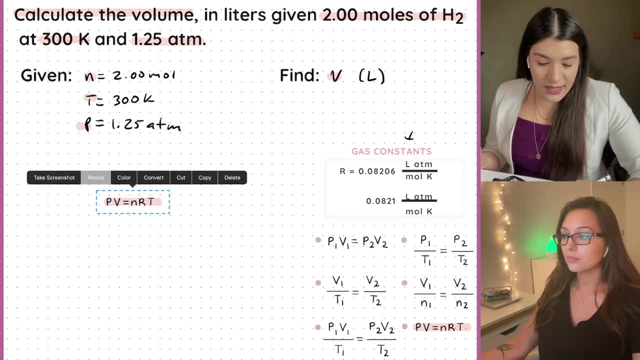 we don't have two volume, two temperatures and so on on. Well, it's this last one, the ideal gas law. So I know that I'm going to use this, And R is actually it should be given to you, And you're either going to see it like this top one. 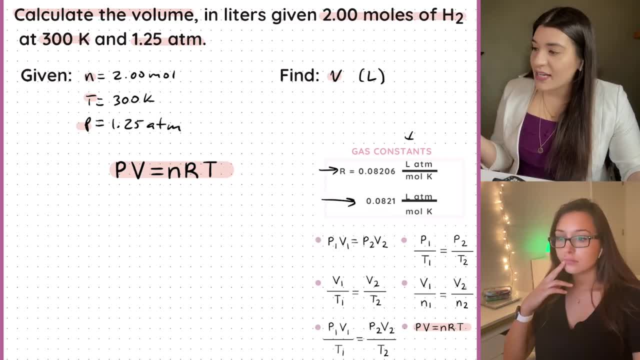 or this bottom one. Both of them are the same, So still the same thing. One is just rounded, The other one isn't. So I'm going to use, I'm going to use the bottom one. That's kind of the main one that I always use, but it honestly doesn't matter, So I'll put in pressure. 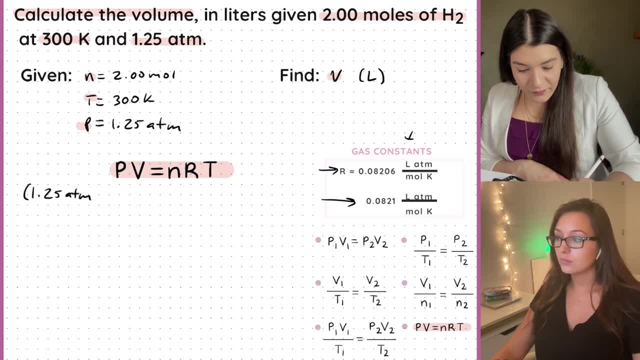 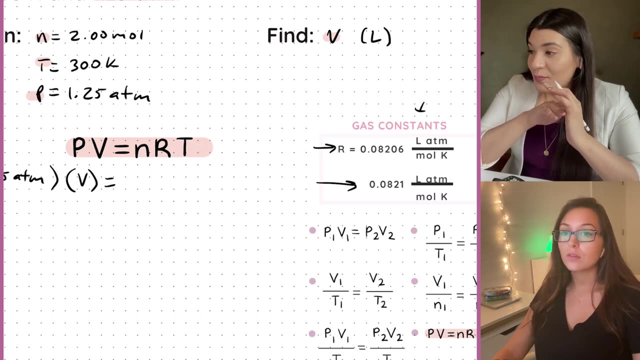 So P is 1.25 atmospheres. I'll put in we actually are solving for V. And before I even continue, I realized one thing I wanted to mention. So the units for all of this is totally fine because of the gas, gas constants units already. So if you notice the units for our R. 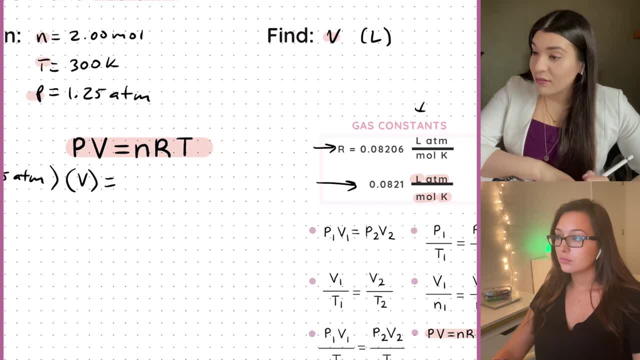 it's already in liters, atmospheres, moles and Kelvin, And this is kind of like when we were talking about the gas constant, we were talking about the gas constant and we were talking about the gas constant and we were talking about the gas constant and we were 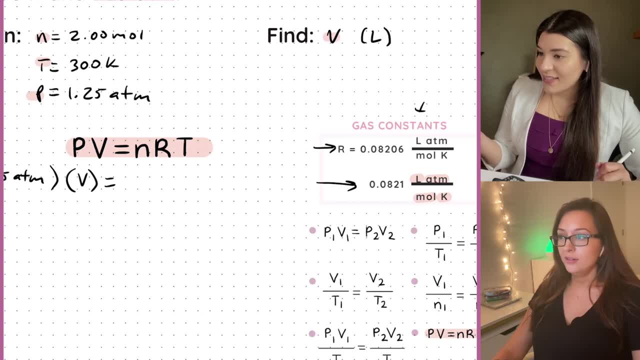 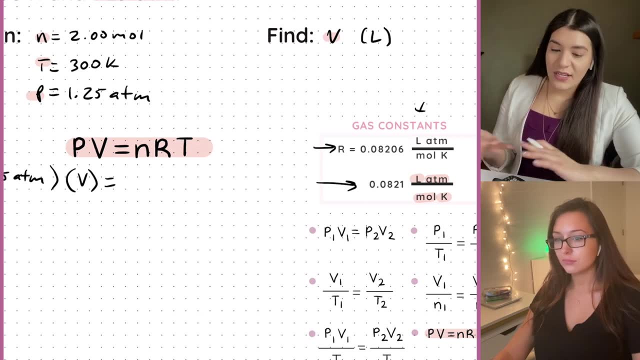 talking about calorimetry with the specific heat capacity, where all of the units have to align or be the same as the specific heat capacity. It's the same sort of concept here with the ideal gas law. Like, you want your moles to be in moles, right, We want that to be in moles, You want. 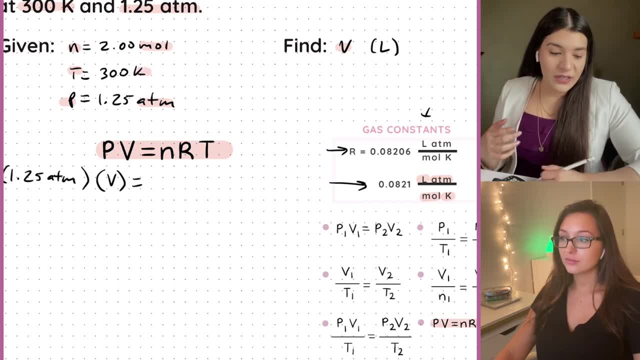 your pressure to be in atmospheres. We always want temperature to be in Kelvin and we're going to want our volume to be in liters, And that's why all of this is totally fine. However, if we were talking about the gas constant, we would have had to have converted this to atmospheres. 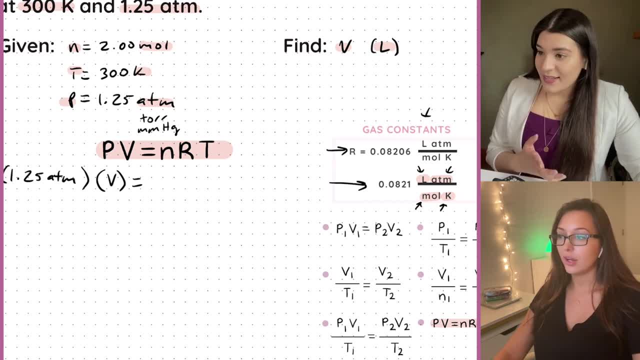 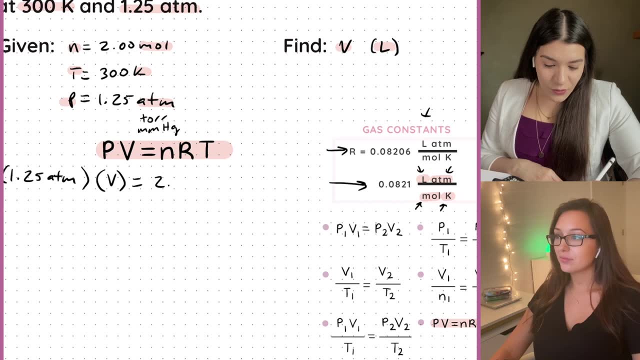 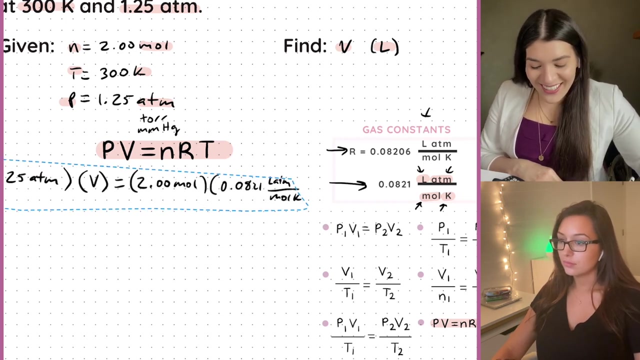 just to match the gas constant. Does that make sense? Okay? Yes, Yeah, Same principle as before, It's just a different formula. Yeah, exactly So cool. Two moles, And then next our gas constant, So 0.0821 liters atmospheres divided by moles Kelvin. Sorry, I used to. I had to. 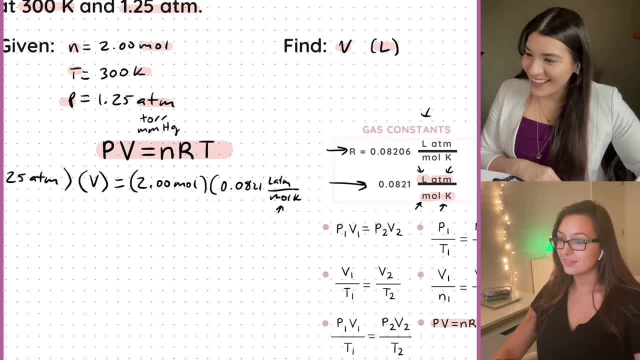 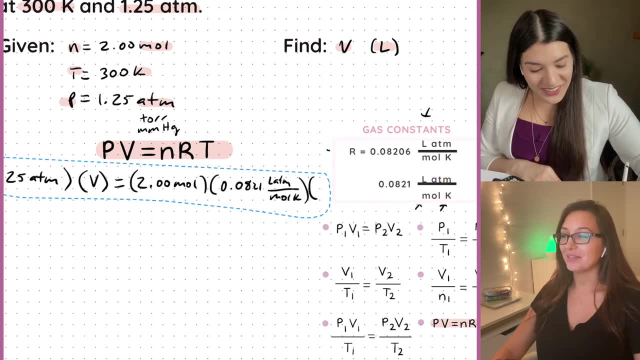 a student who would always think that this said molk. I just like that. That's what they would always say. I don't know, Just reminding me of it right now. That's funny. It sounds like something I'd say. It's very cute. Yeah, He was a high school student, And every time they're like